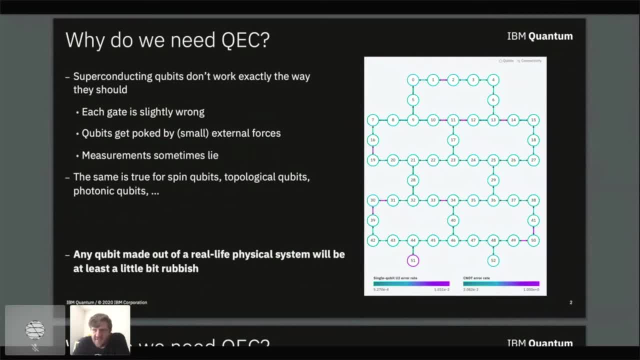 will get perturbed by external forces. as an interaction with the environment is what we call this, and the measurements that we make sometimes lie. Sometimes it's a zero and you measure it and it tells you it's a one. Now, this isn't something that's uniquely. 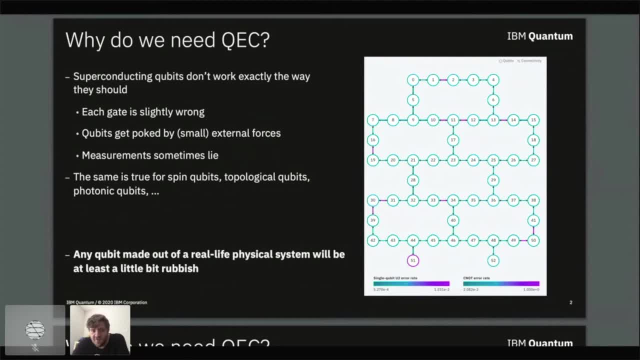 true for superconductors, It's not true for the quantum-computing qubits, but the same is also true for all other ways that you might imagine to make a qubit out of some physical system. So there's other ways of making qubits, such as spin qubits, topological qubits, photonic qubits and all. 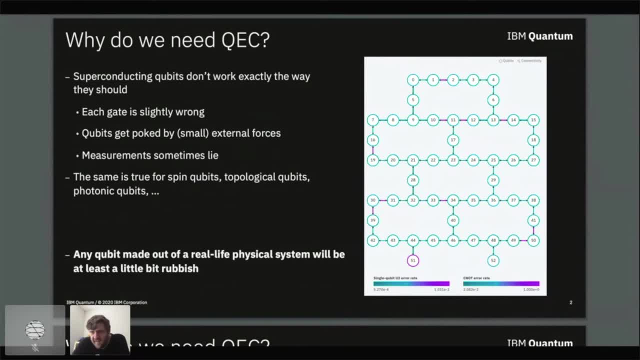 other kinds of things. This is just sort of random words for you at the moment, probably, but there are many ways that people have tried to make this thing that you've been learning about for the past few years. The first way is to make it in real life, and they use different physical systems to 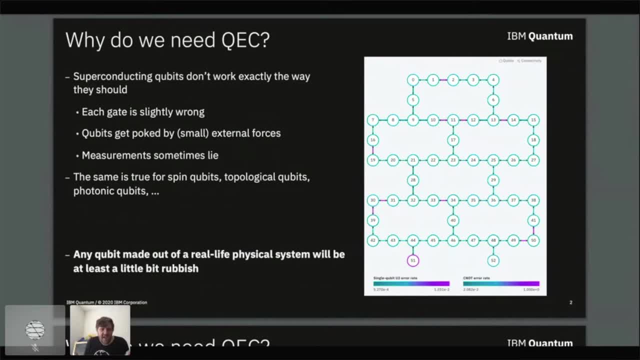 do that and anything that they use, it's always going to be a little bit rubbish. There's no way of getting around that. We can make it as good as we can and we can reduce these effects as much as we can, but they will always be there to some degree. and when you're thinking, 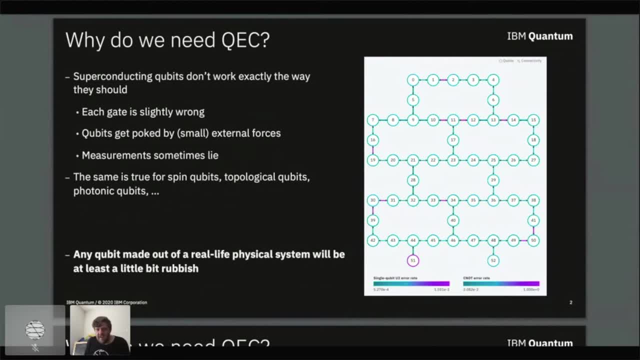 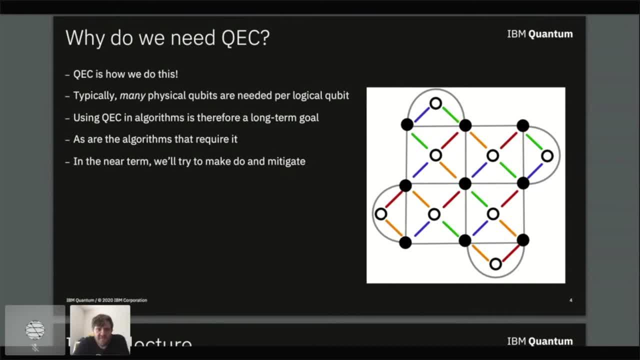 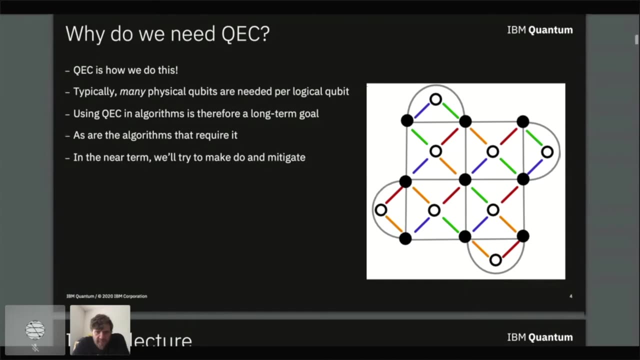 try and use logical qubits, but we'll use the physical qubits that we have and just try and mitigate errors by less formal techniques than we do for quantum error correction. So this is an overview of why we need quantum error correction. What we'll do in the rest of 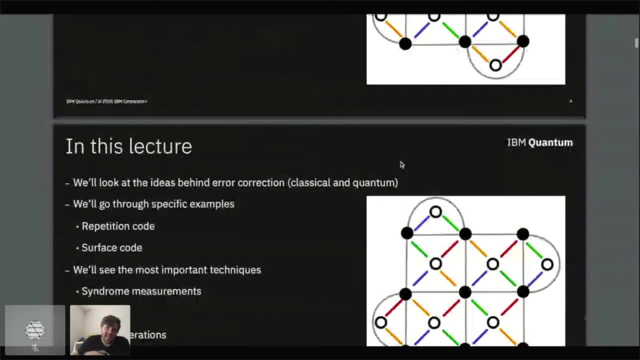 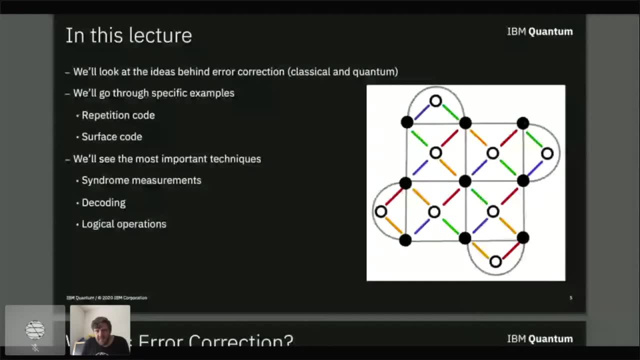 this lecture is look in detail at the ideas behind error correction, both classical- although we won't go into the real depths of classical error correction theory- And we'll also, of course we'll, look at quantum error correction. For this we will go through two specific examples of ways. 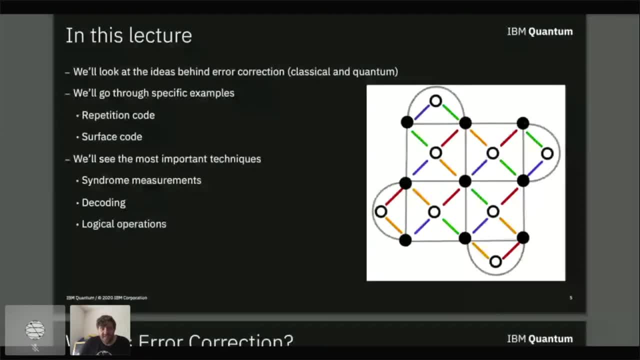 how to do quantum error correction. One is the repetition code, And the reason why I want to tell you about the repetition code is because it's the simplest quantum error correction code, So I think it's the best example. But the bad thing about 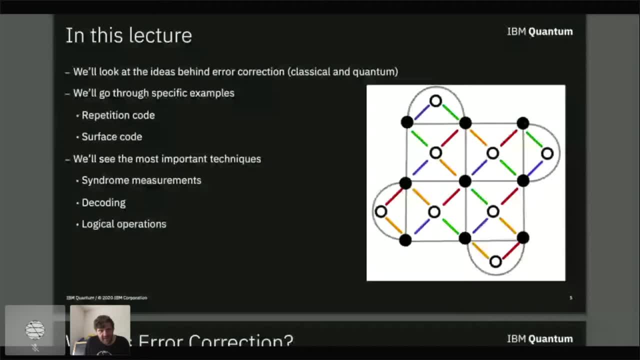 the repetition code and the reason why that's not the only one I'm going to tell you about- if it doesn't actually do everything it needs to do in order to help us build proper logical qubits, And so for that we're going to look down at the surface code which fixes the issues. 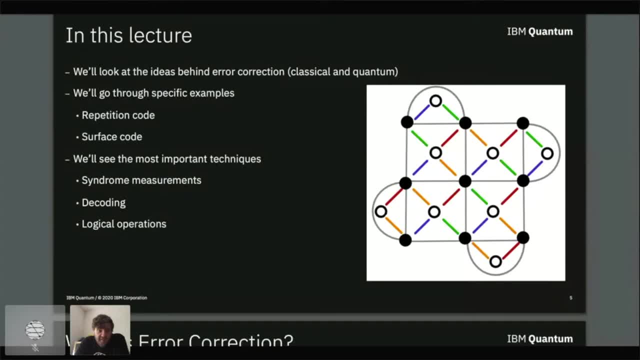 in the repetition code And the surface. there are many ways of doing quantum error correction, all usually called something followed by the word code. But the surface code is is, I would say, the the most popular, the one that people think is most likely to be used in the 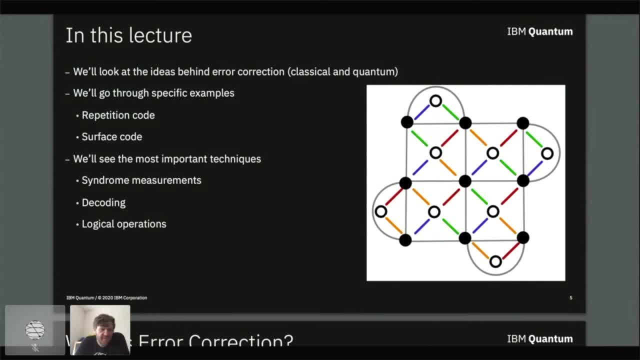 end to do quantum error correction, or at least some variant thereof. In this we will see in both of these codes all of the most important techniques which are relevant for all forms of quantum error correction, which are syndrome measurements, decoding and logical operations, and these will mean nothing. 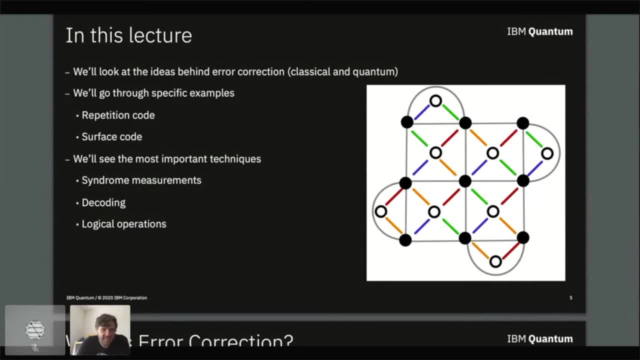 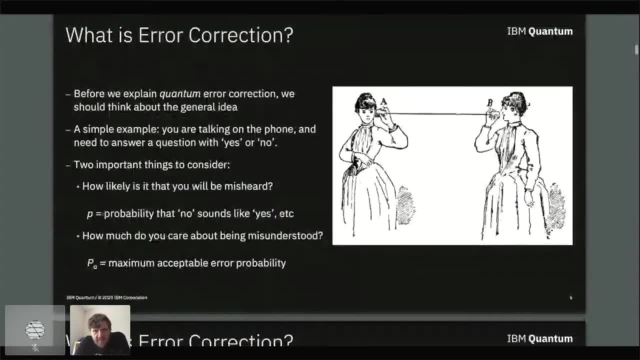 to you at the moment, but the idea of the lecture is at the end. they will mean something to you. So we'll begin by just looking into what is error correction as a whole, what is even the concept of error correction, and for that we can. 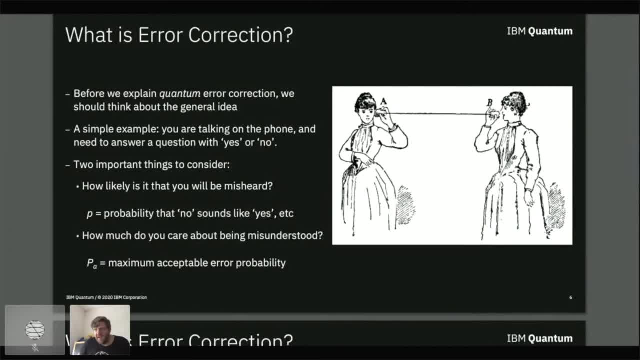 think of a classical example. in fact, we can think of a very, very down-to-earth example of people talking to each other. so say, you're talking on the phone and someone asks you a question, you need to answer that question with a bit of information you need. 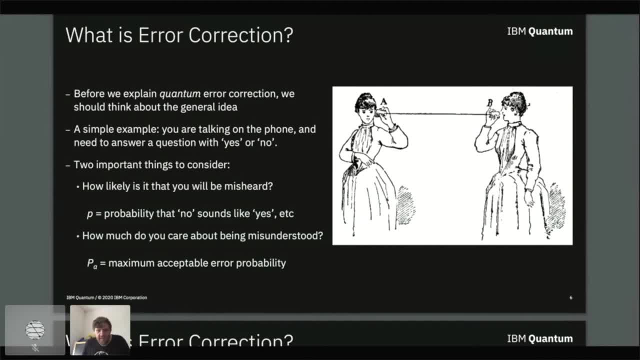 to answer that question in binary so you could say zero or one if you were a computer. but usually when humans talk in binary they say yes or no, so you need to answer a question with yes or no. maybe you're being asked: do you want pineapple on your pizza, yes or no? and there's two important things. 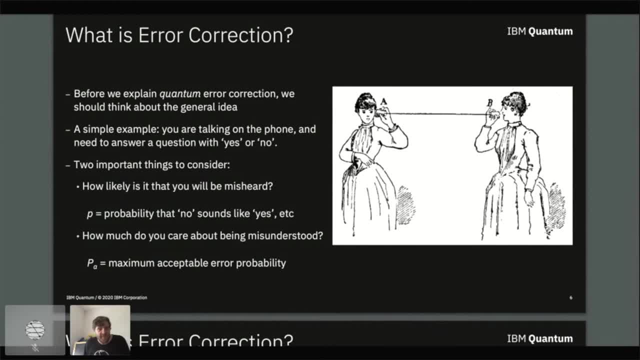 now to consider how likely it is that you will be misheard, so maybe it's a perfect line. there's no flaws in the in the line at all. you know that everything you say will be heard in absolute detail. so in that case, if you- uh, if you don't want pineapple on your pizza, you can just say: 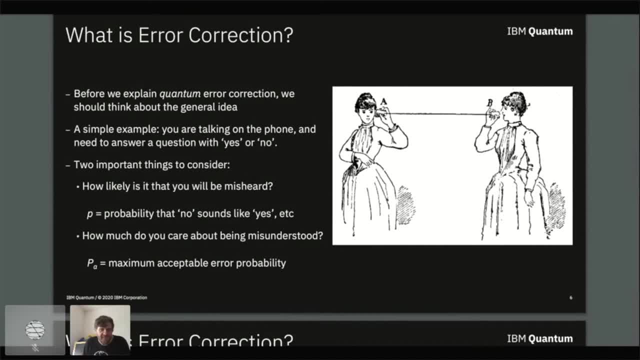 no, and you'll know that they have understood that. um, but maybe it's a noisy line and if you say no, they're not really going to hear. they might think: what was you? was that? yes, i'll put pineapple on, um, so what is the probability that you're going to be? 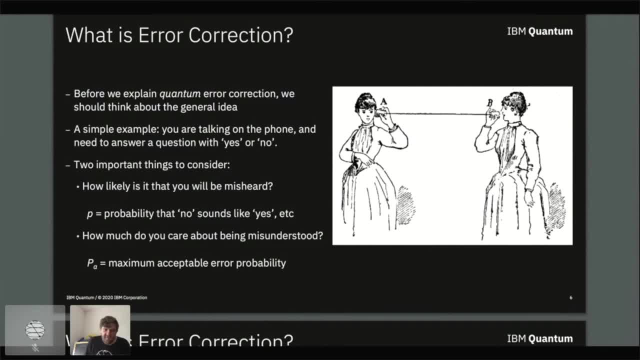 misunderstood. and also, how much do you care about being misunderstood? because there's there's no way that everything can be perfect. this is just a fact of life, so there is always some probability that you're going to be misunderstood, like one one in a trillion billion chance that aliens 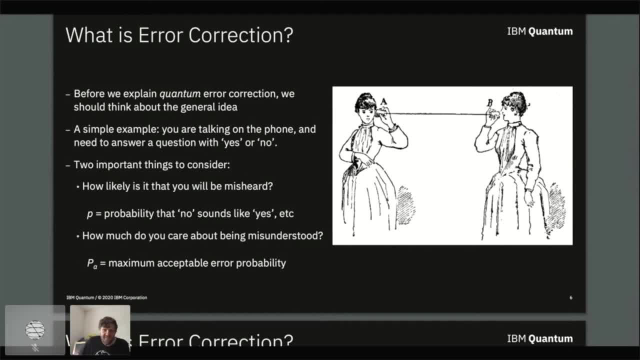 are going to intercept your message and so any longer you think about pineapple, maybe for 20 minutes or one hour, but hopefully you don't really stop. just flip it to be annoying. um, so there's always going to be some probability, something's going to go wrong and you can think: what is the what, how much? 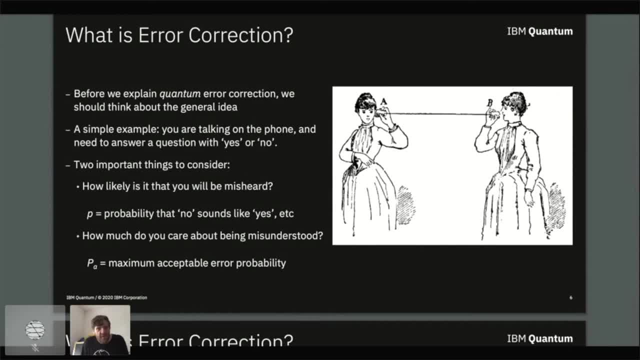 do you care? so maybe you don't really care whether you have pineapple or not. this is not an issue that affects you. you know that. you know that some people get very passionate, but you particularly don't care, so then this would be, uh, quite low. but if you have very strong opinions on 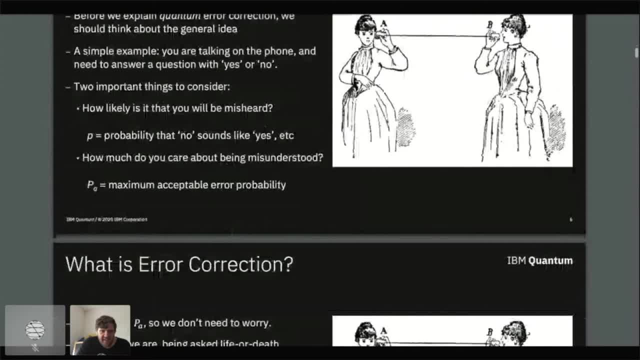 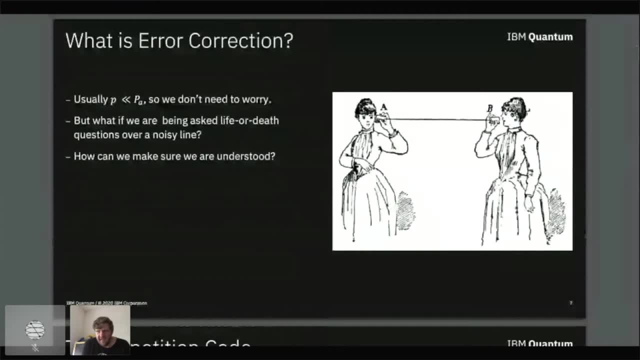 you can think. well, if the probability of getting misunderstood is very much less than the acceptable probability, so it's much less likely to be misunderstood than the limit that you care about, then you don't really need to worry. You'll just say yes or no, whatever. 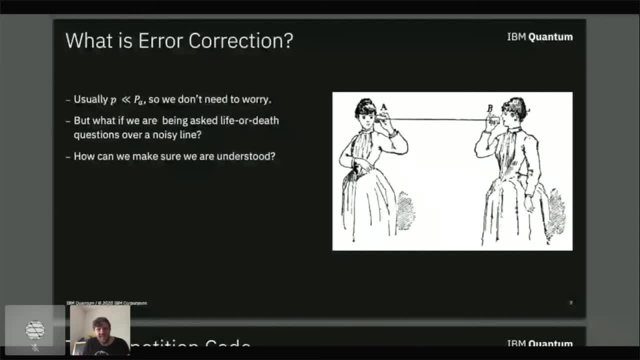 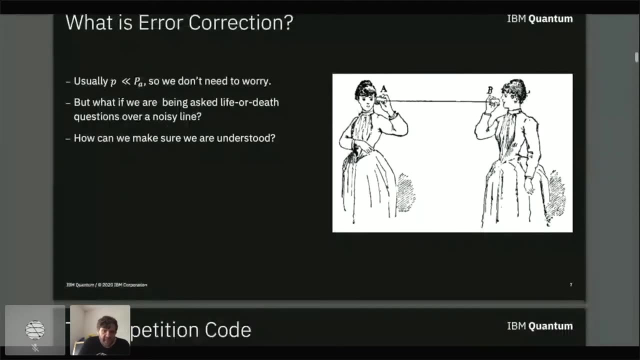 But if you really want to get your message across, then you will have to do something rather than just saying yes or no, in order to ensure that your message really is understood, despite the fact that the line that you're using is too noisy, And what you would probably do. 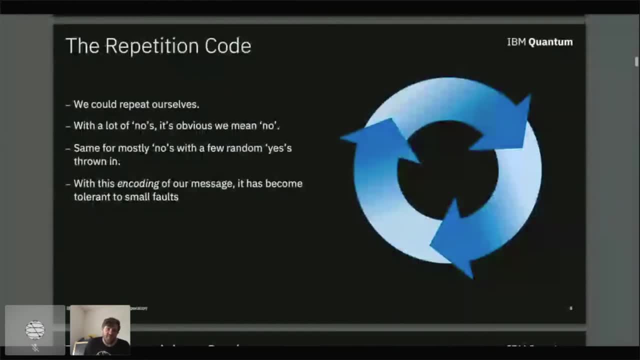 without even thinking is repeat yourself. So if you really wanted pineapple on your pizza, you would say yes, yes, yes, yes, yes, yes, yes. Are you kidding me? Yes, of course. And once a person has heard that, then even if there's some interruptions in that signal, 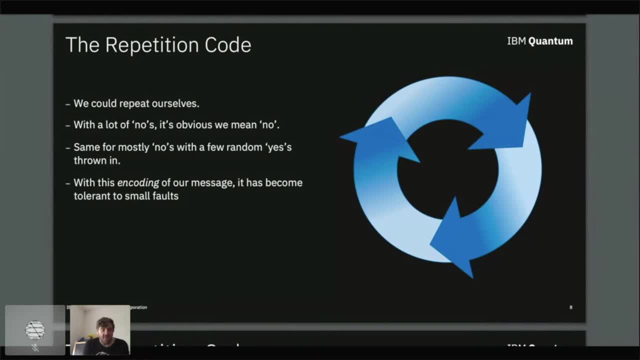 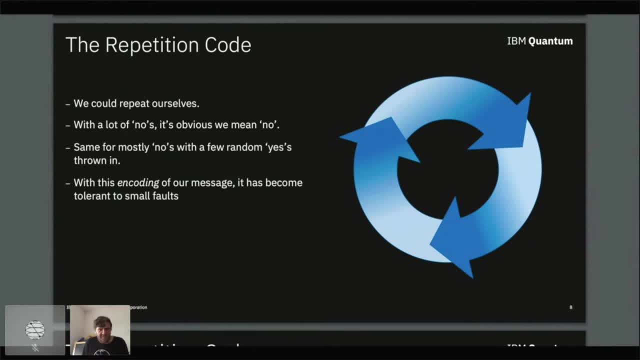 is a way of encoding our message. It's taking our message and expanding it to something bigger, Such that it becomes tolerant of small faults. And in this case, it doesn't matter if a few of those words that you're saying get discarded, if they just turn into noise or if some AI. 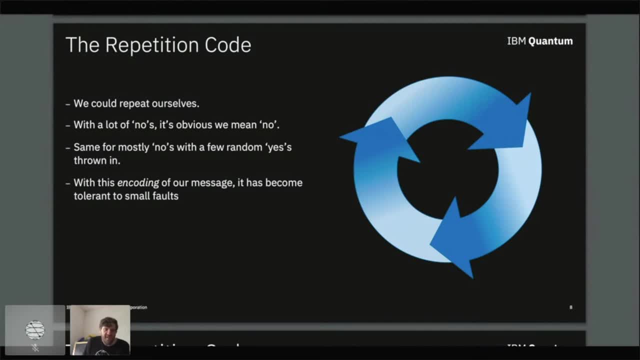 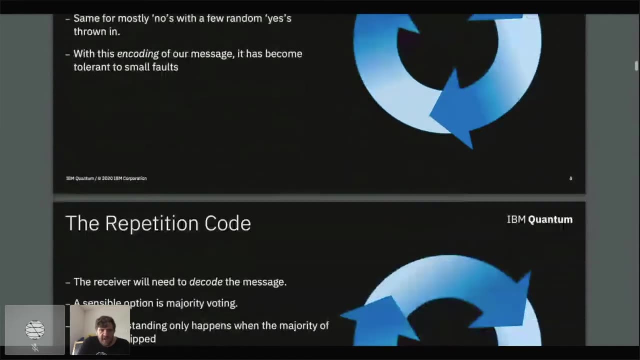 misidentifies them and turns them into the other thing or something, It doesn't matter, Your message is still getting through, just because the way you have encoded it in repeating it, has made it more tolerant to small faults. Yeah, Then, so that is the encoding step. You are taking your information: a yes or a no? 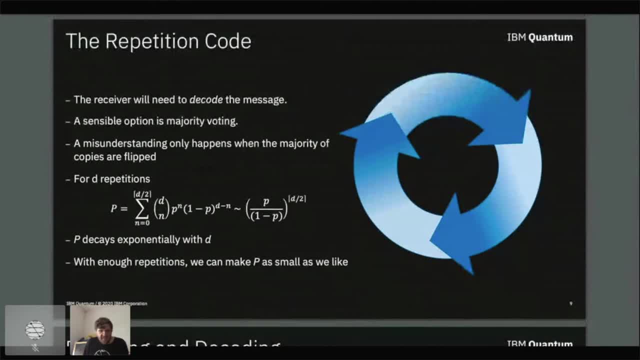 and you are encoding it somehow And your yes becomes yes, yes, yes, yes, yes. Your no becomes no, no, no, no. But at the end the receiver has to decode the message. Now, in this case it's fairly easy, because your message is just many copies of exactly. 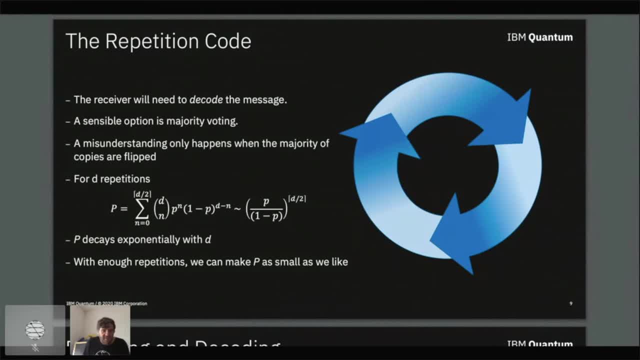 what you want to say In error correction. sometimes the way we encode it is something more more abstract. So if you receive an encoded message, it's like receiving an encrypted message. It makes no sense if you don't know how to unpack it. So it can be that sometimes. 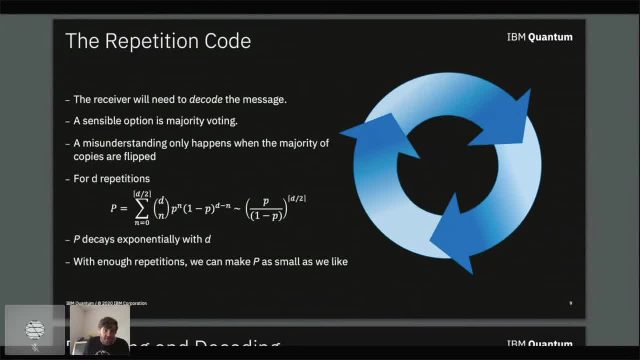 we encode a message in that sort of form in order to make it more robust against noise. But in this case it's kind of easy. What you could do is majority voting. So if the receiver received a number of yeses and nos, then if they receive more yeses than nos, then they'll. 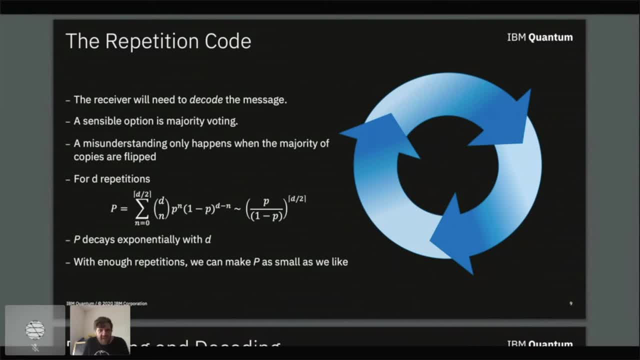 probably think: well, that sounds like a yes. Let me get out the pineapple. In this case, a misunderstanding will only happen when the majority of the copies are flipped, which is possible but it's unlikely. So if you say yes instead of yes, you say: 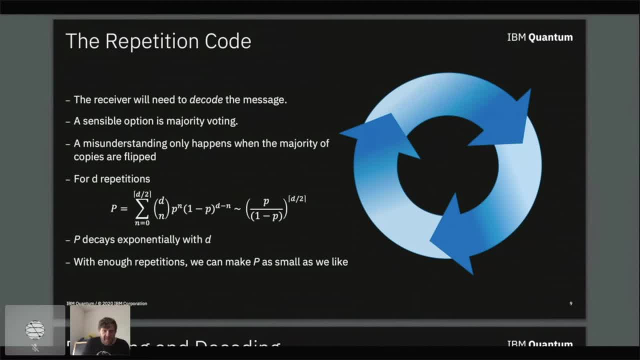 yes, yes, yes, And there's some probability of one over 10, that one of those words gets messed up. Then the probability that one of those words gets messed up is on the order of one over 10.. The probability that two of those words gets messed up is on the order of one in 100.. So most 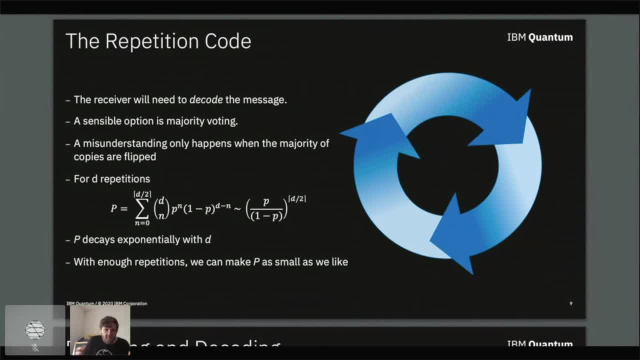 of the time, your yes will be yes, yes, yes. On the order of one over 10 times, your yes will be well, yes, yes, no, and also for yes, no, yes and no, yes, yes, So sometimes, 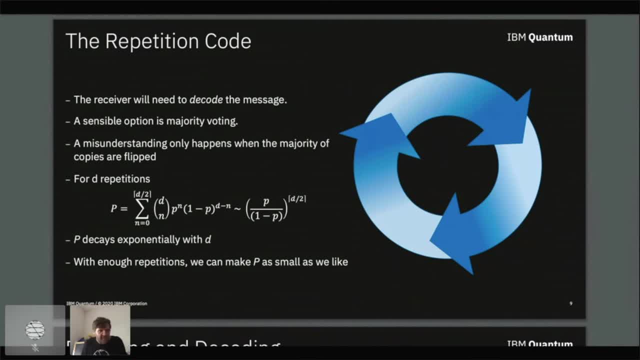 that'll happen, but that's okay. People understand from the majority that you're saying yes, But about one in 100 times you'll get something like two of those yeses perhaps being flipped to a no, which is quite a weird error model, to be honest, When you're talking on a call. 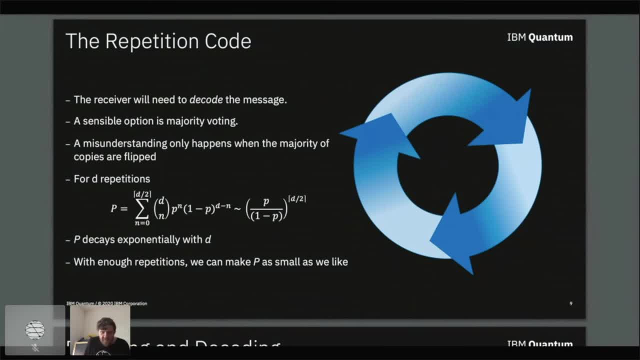 your words don't usually get turned into other words, But let's assume it's a simplicity About one in 100,. there's a chance that, even though you say yes, yes, yes, because there's been two error events, it sounds like yes, no, no, And the person who is 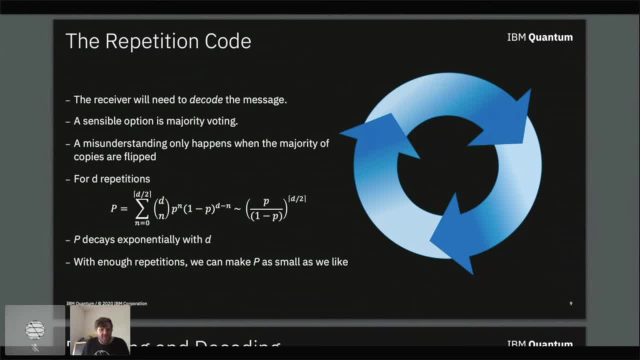 who is decoding this will think that you said no even though you said yes. So that is a probability of something being incorrect, And the probability that that will happen is the probability that at least the over two errors happen. So actually there's an error in. 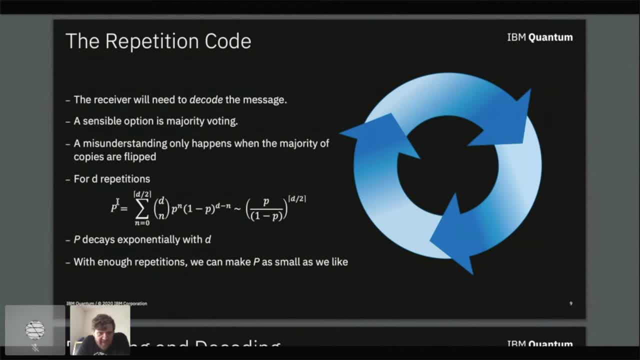 this equation, but this should. this is the probability that something goes wrong. I'm not sure if, actually, you can see me highlighting this, because it's only going to be one of the only capture in Chrome, But this is the probability. You can see it, Okay? So this is the 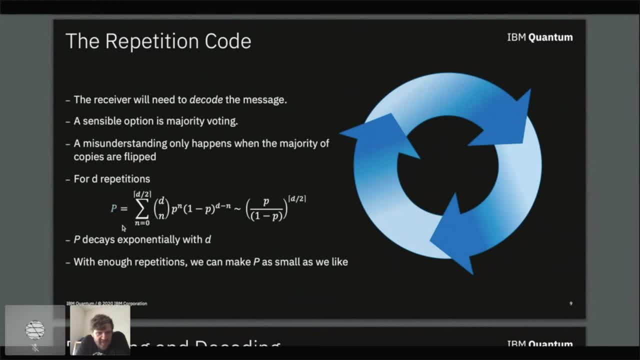 probability that the person trying to decode your message decodes it incorrectly, And it's a sum over all of the possible ways that they can decode it incorrectly. So it should be the sum from D over two, which is half of D is the number of times you repeat. So D over two is half the. 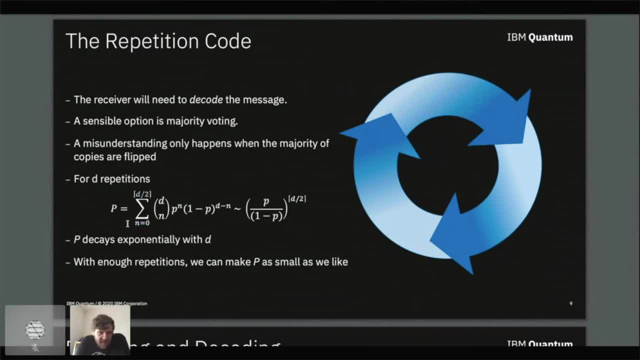 number of times you repeat and then sum that. So it's all of the different ways that you can have half or more of the errors flip And the probability of this scales well. it's the probability that a flip happens to the power of. 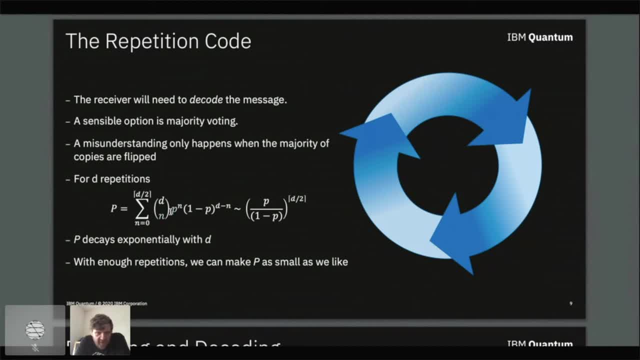 the number of times you might get a flip And there's binomial coefficients and all that. But really it's just, it just scales with the kind of like the probability that a flip happens to the power of the number of times you might get a flip. So it's all of the different ways that you can. 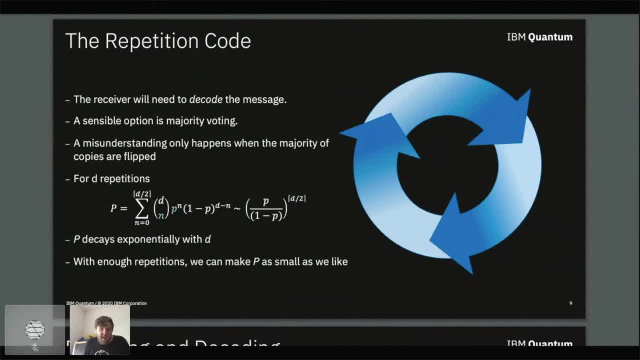 get a flip. So it's all of the different ways that you can get a flip. So it's all of the different ways of the minimum number of flips which is problematic, which is half, So the probability of something going wrong. when you repeat three times, it scales a sort of p squared, because p is 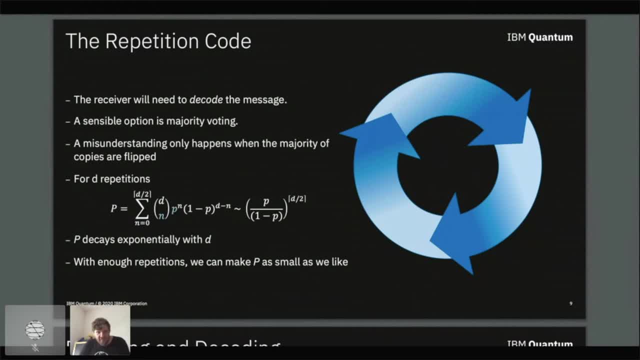 the probability that something is going to go wrong with each of your yeses or nos. And it's squared because you need to do it two times to flip the majority for three, But if you repeat it five times it'll be p to the three. 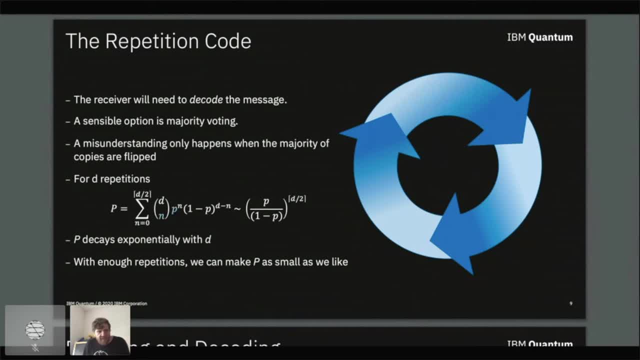 So it's all of the different ways that you can get a flip And that's the minimum number of flips. repeated it 101 times, it would be p to the 50. So the probability that the majority gets flipped decreases exponentially as you increase the number of repetitions. So as certain as you want to be, 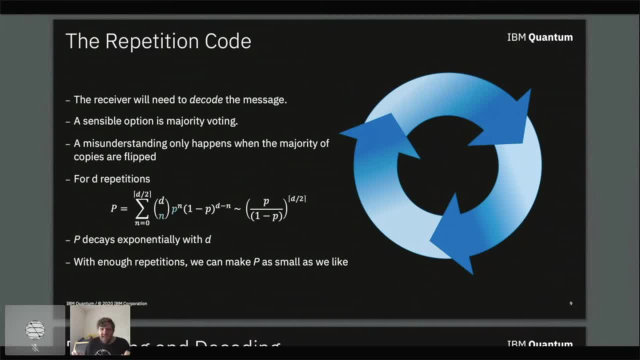 that you do or do not get pizza. sorry pineapple on your pizza. you can just make sure that happens by repeating yourself enough times, And I think this is something that, intuitively, we kind of know. anyway, If we really don't want it, we would be saying no, no, no, no, no, no, And I don't know why I picked. 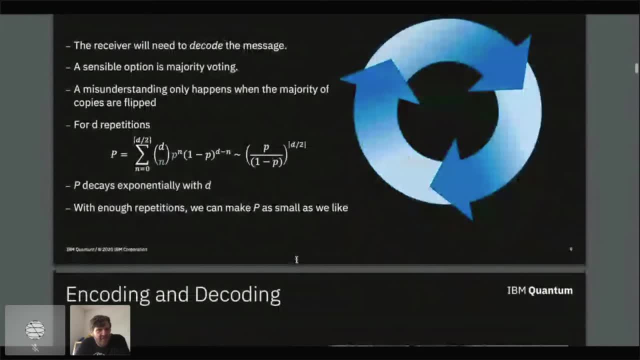 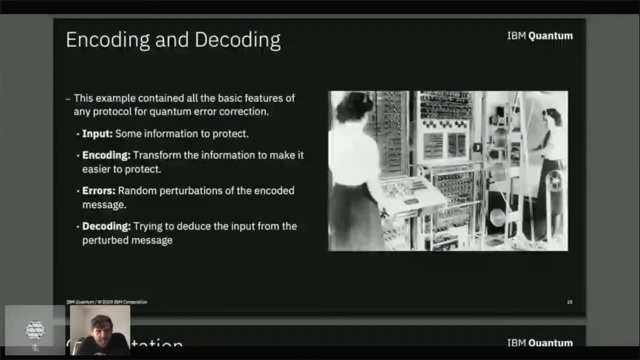 this pizza example randomly, because I don't have strong opinions on pineapple, on pizza. I know perhaps that's going to annoy some people, but there you go. Okay, so this is a simple example and it in no way involved any quantum yet, but it has. 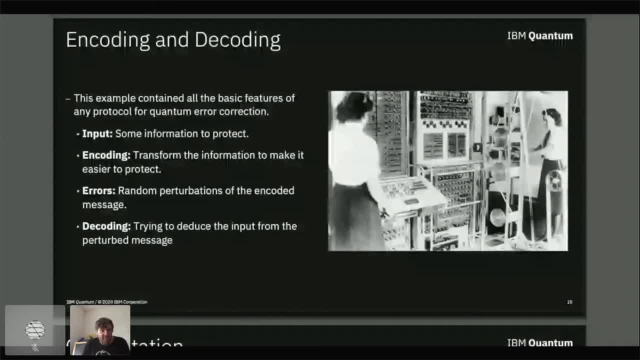 the very basics of quantum error, of quantum error creation or error creation, any kind of error creation. So it's basically a process that we have to go through and what we're going to do is actually step of encoding and decoding. So we have some input, so some information that we want to protect. 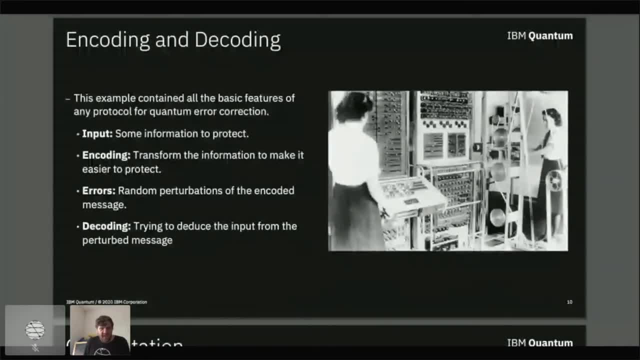 And then we put that through a process of encoding. We transform it in a way- usually by making it bigger so it covers more information, more bits or more qubits, and we transform it in a way that makes it easier to protect. And then a process comes along which causes errors. 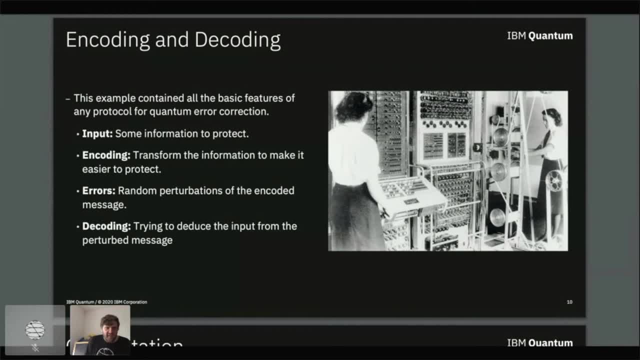 So these are perturbations of the encoded message. So after that we don't have exactly the encoded message that we started off with. It has been messed up a bit. And then we have the decoding process, which is basically solving a puzzle. 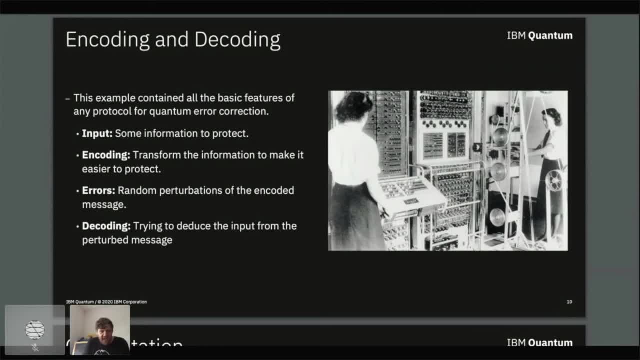 We are given this messed up encoded information and we're told some errors happened, but we don't know where. Try and figure out the clues of where the errors might have happened, to undo them and deduce the original message. So that is basically the puzzle at the heart of quantum error correction. 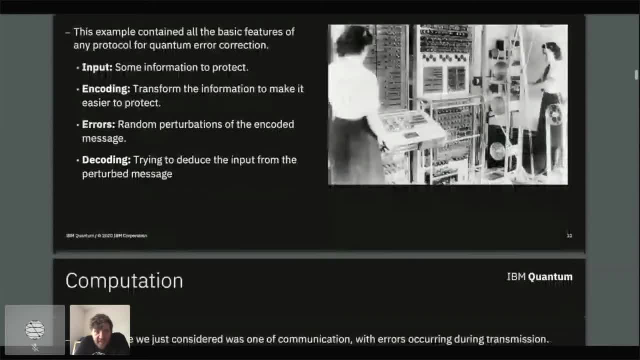 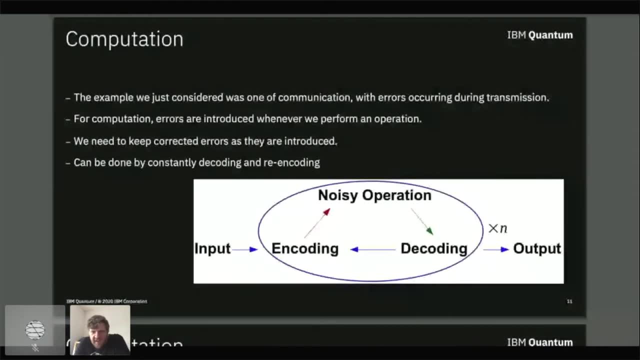 In fact, I made it into a puzzle game a few years ago called Decode Cooper, which I think might even still be on the App Store, but it's not something that I am really too much with anymore, But it might be fun as a game if you want to play something. 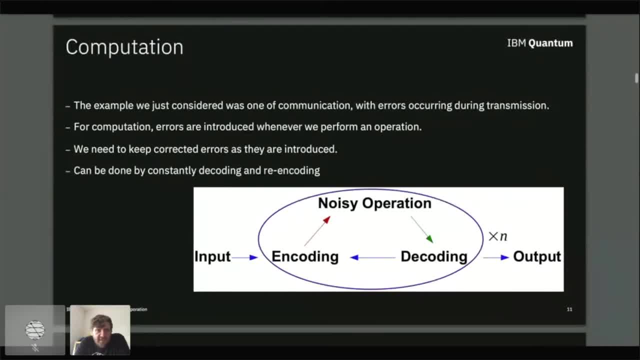 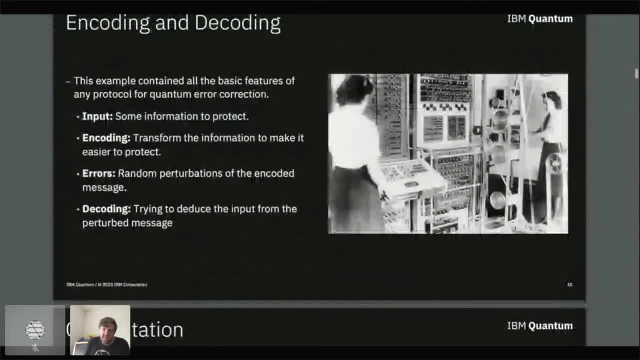 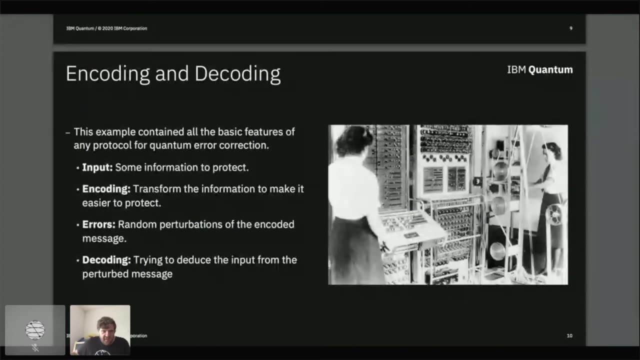 Okay, So that is well. this description is actually more geared towards error correction in the telecommunication where you want to send a message, So you encode it. errors happen along the way. you decode it, you get the message done. 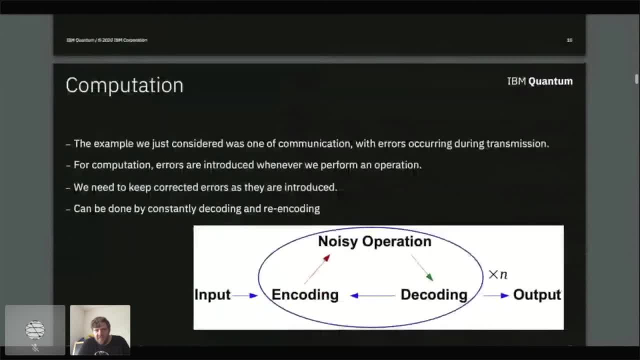 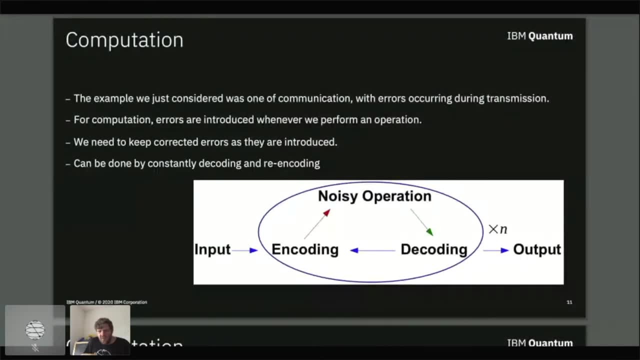 This is not really the kind of error correction that is important for us, because we are doing computation And in computation we want to do error correction, which encodes our information at the beginning and then we do a computation on that encoded information. 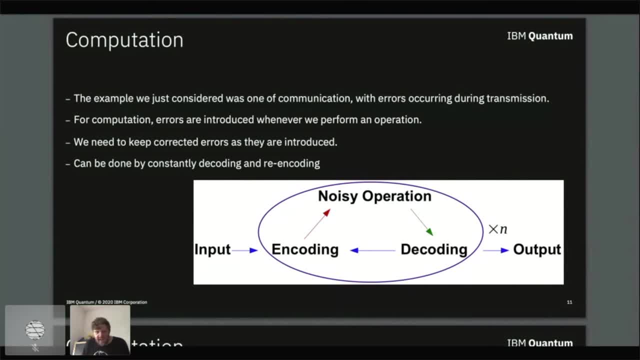 We want to keep it encoded so that throughout our computation, any errors that happen, we can fix them. When we do operations in our computation, any errors that happen in those operations, any errors that we introduce just by the fact that we are doing an algorithm, we can fix. 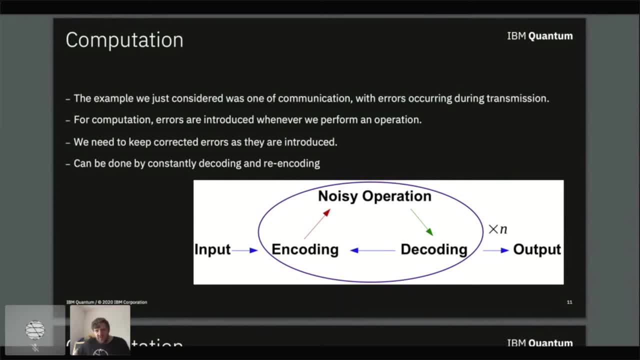 them, And then, at the end, we do decoding to get an outcome, Although actually it's not exactly that simple, because leaving everything to the end in terms of decoding is not a good idea. So what we'll really be, What we're thinking of doing, is having our input, which is just our all zero state, probably. 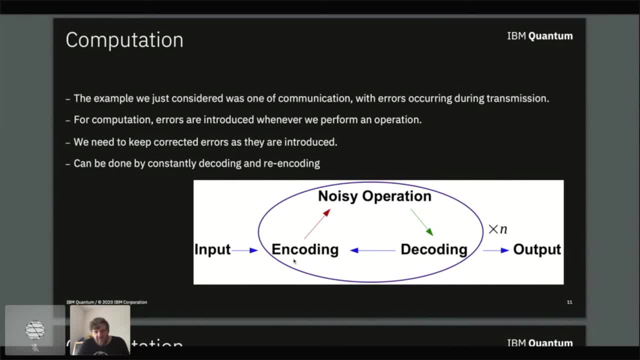 and we encode it in some way And then it keeps on going through a process of being: Maybe we're doing an operation and that's causing noise, or maybe a qubit is just idle for a while and it's picking up noise from the environment. 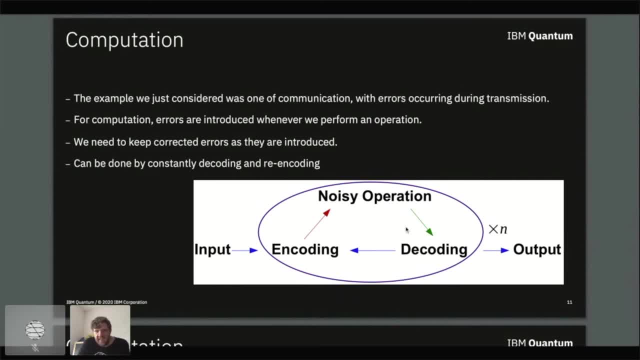 Whatever's happening, noise affects it, and then we need to fix that noise. So we decode and we re-encode. more noise happens, decode, re-encode. more noise happens, decode, re-encode for as long as it needs for us to do our computation, and then we 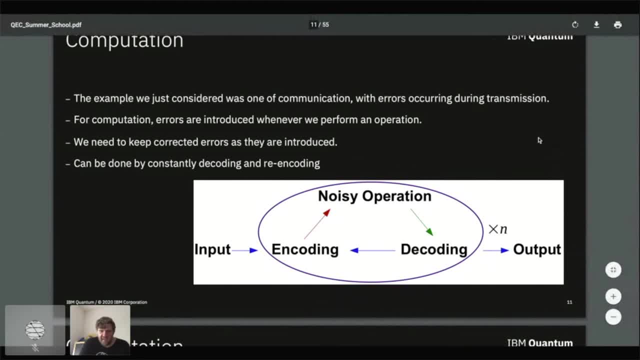 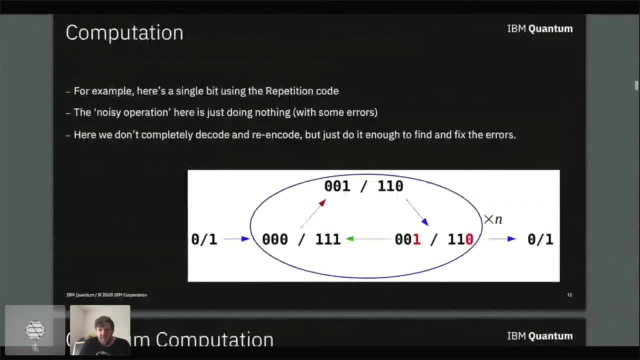 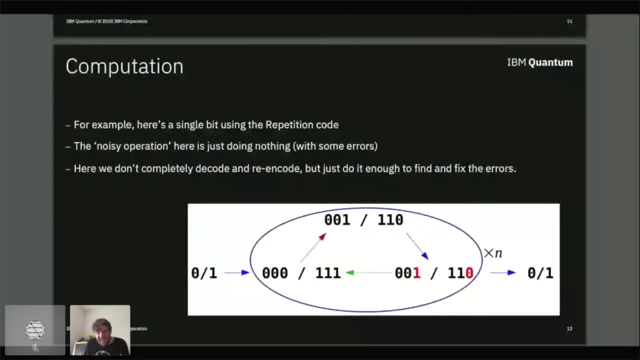 get an output. Although here I said we decode and then we re-encode, that is not actually fully true, because if we decode, then we get back down to an unencoded state, which is we have encoded exactly because we want to protect ourselves from the effects of errors. 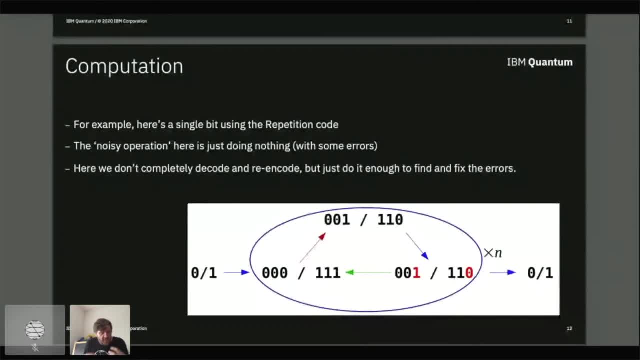 So once we decode, then we're back. We're back to being vulnerable again. we don't want to be in that state, So we don't want to. We want to do some decoding to fix things a bit, but without actually going back to. 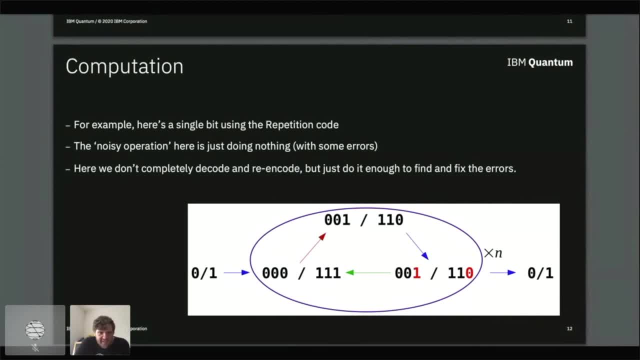 our unencoded state. Now let's give you an example so that sounds less abstract. So let's just think of a single bit encoded using the repetition code. So what we could have here is that we have either a zero or a one. So 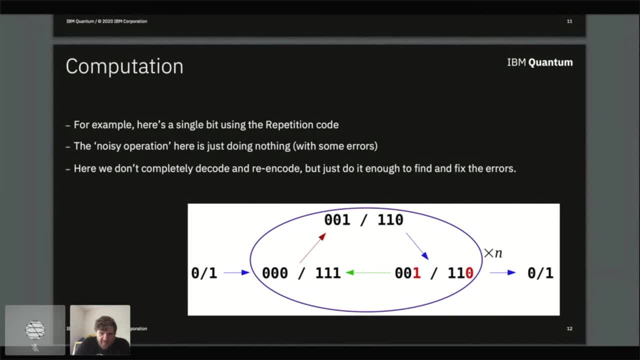 And if we had a zero, then we would, in the repetition code, repeat this three times to get zero, zero, zero. And if we had a one, we would repeat it three times to get one, one, one. And then let's say: 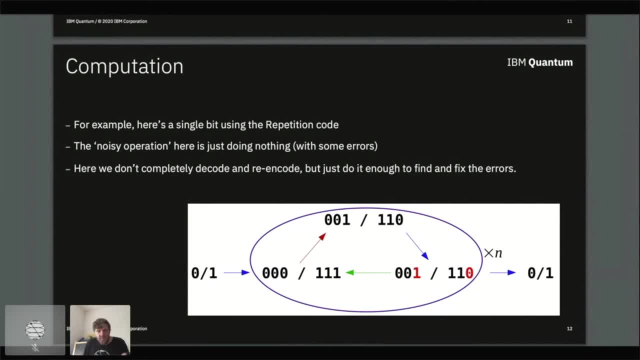 And it goes through some noisy process. We're not going to try and do an operation here. We're just going to consider the idea that the environment comes in and causes a bit to flip, And let's say that it's the last bit that flips, just as an example. 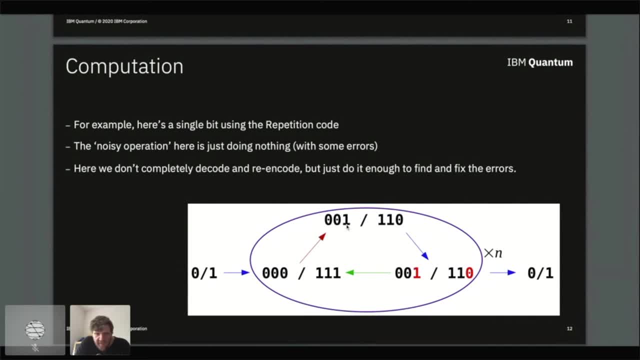 So our zero, zero, zero in that case would become zero, zero one, because the last bit has flipped, And if we had an encoded one, our one, one, one would become one one, zero. So then we can look at that and we don't even need to decode that. 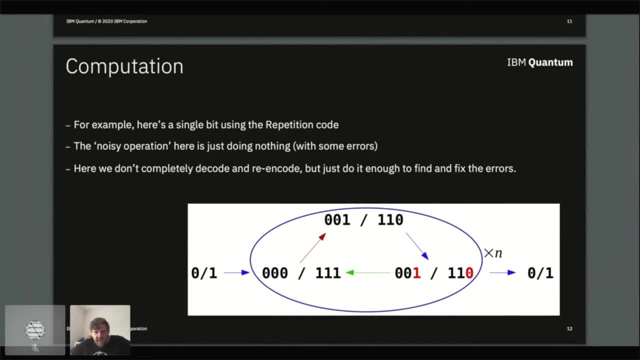 We can look at that and think: well, there's two zeros and a one. That one is out of place, Probably it should be a zero, And then we can identify that because it is Okay, It is not the same as the majority, that it's probably because of the majority voting in. 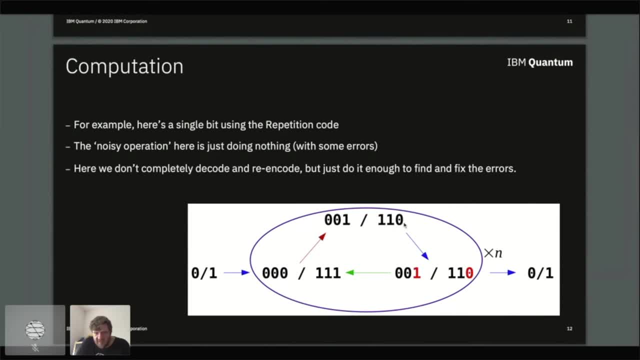 this code the error, And similarly, if we found one one zero- we'd see similarly that this one is out of place. So we identify that as a problem and then we can fix the error just by flipping that bit. 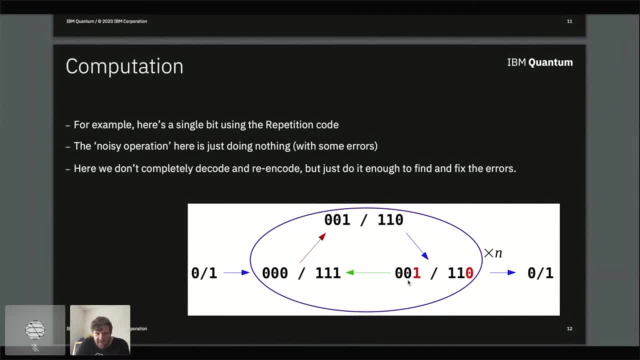 So we can flip the last bit and then, whether we encode the zero or a one, it fixes it. So we're going to do it, So we're going to do a process of trying to find while it's still encoded. we're going. 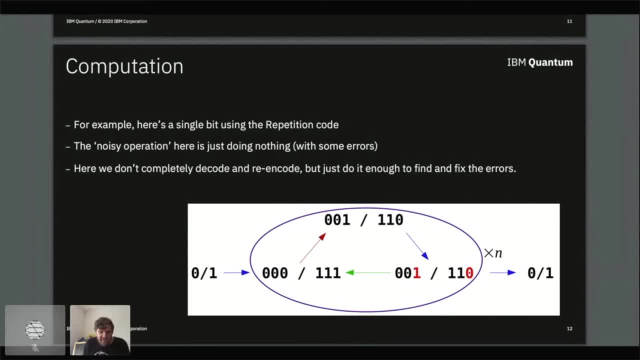 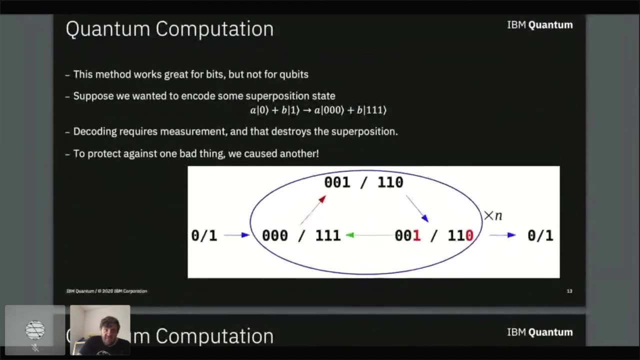 to do a process of trying to find hints about what errors have happened, so that we can keep on cleaning up our encoding while we're doing a computation. Okay, So this particular method with the repetition code would be fine for bits, but it's not. 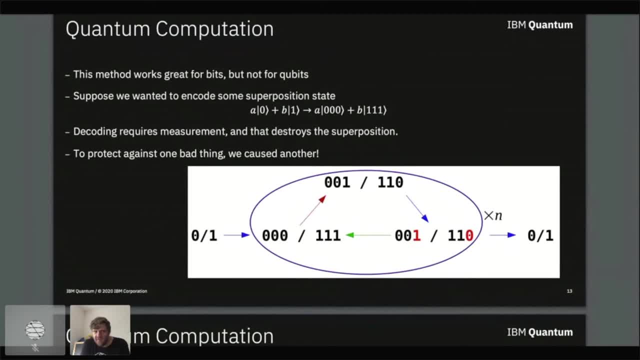 so great for qubits. In fact it's not even great for bits, because it's kind of not a very. There are certain ways in which the repetition code, even for bits, is not a great code, But that's mostly due to overheads. 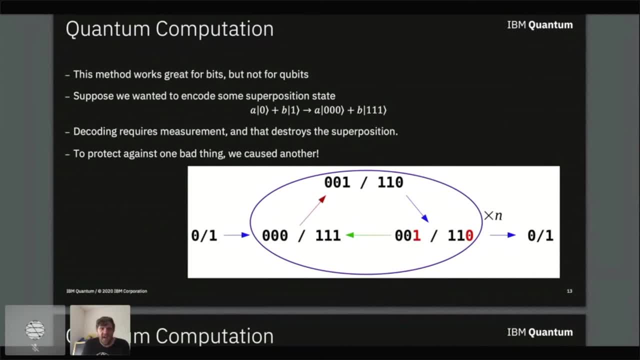 We won't go into that though, because that's all classical error correction, But we will go into why it's not great for qubits. So, for example, suppose we did not just want to have a qubit in state zero, or a qubit in 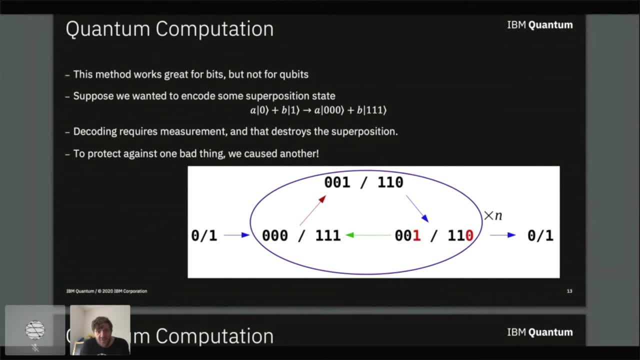 state one, but we wanted to have a qubit in a superscript. Okay, So we would have a superposition state some a zero plus b one. Then, when we go through this process, what would happen? Okay, So, instead of just a zero or a one becoming zero, zero, zero or one one, one we would have. 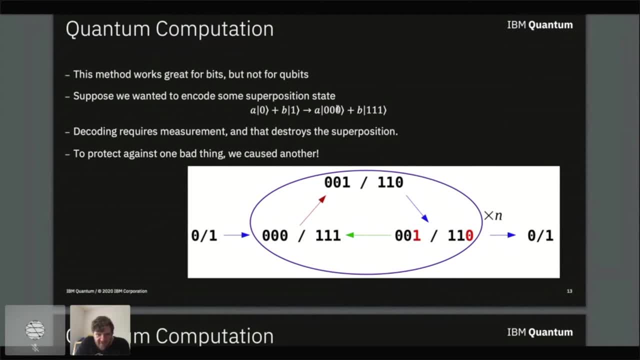 a zero plus b one, becoming a zero zero, zero plus b one one one. So I haven't said anything about what circuit we would use to do that, and you can think about what circuit you could use to do that yourself if you want. Okay. 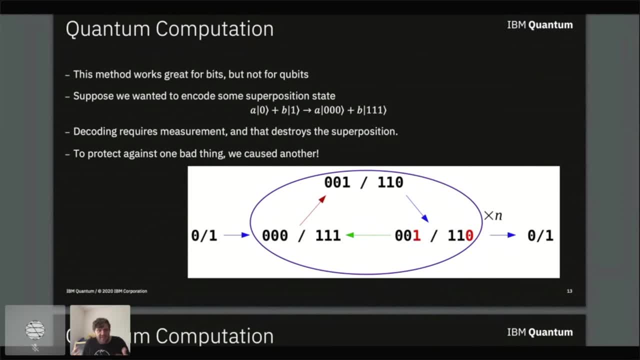 So we would have some circuit which does that encoding, it does that transformation. Okay, Then something happens, An error happens, and again we take the example of a bit flip on the last qubit. Then we would get a superposition of a- zero- zero one plus b- one- one, zero. 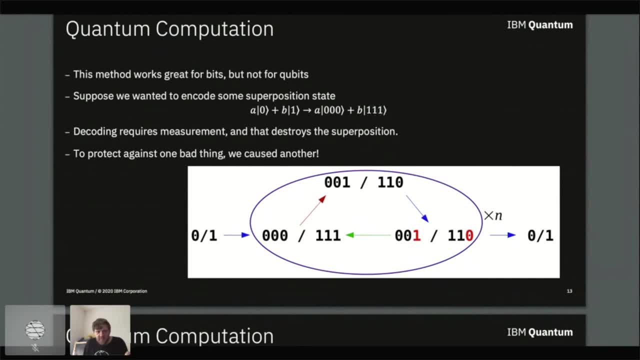 Okay, Then we go to the next step. We look at our qubits, we see what their values are, to see if everything looks okay. So we measure them all And that means that this superposition collapses. It collapses to either being zero, zero one or being one one zero. 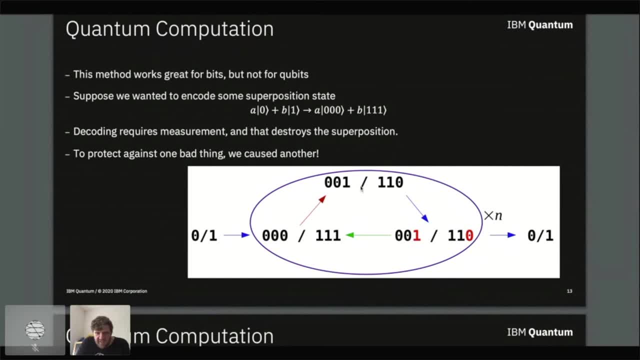 And then we look at that and we say, okay, this one's out of place. whichever it is, We fix it. and we go round and around and around. But the trouble is at that point of measuring the collapse happened. We had a superposition, but as soon as we looked at our qubits we ruined that superposition. 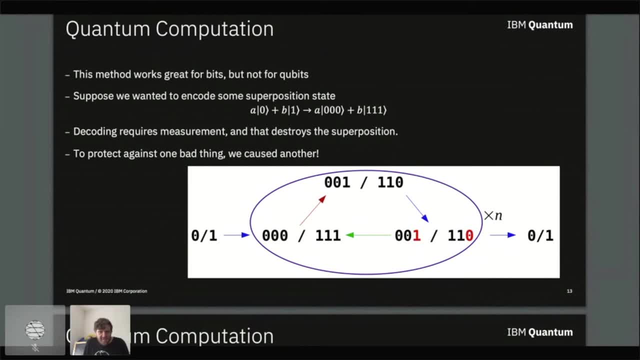 So if we're actually doing a computation which requires that superposition, the fact that, uh, which we're not really seeing in this um, because we've not got any operations in this particular example- we can't see that here, But in general we might have some- we will be doing a computation. that computation would 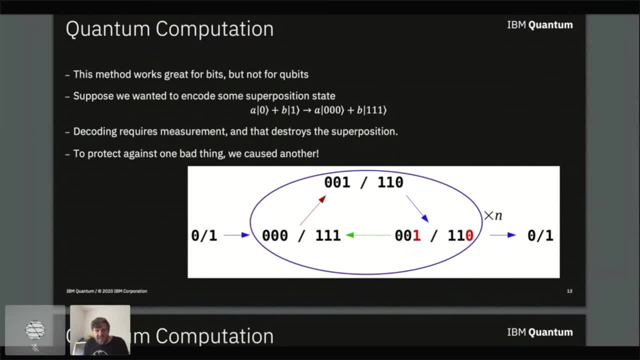 need the superposition to be there. The fact that we have destroyed it by inserting some, some measurements to check up on what's going on is a problem. uh, from the quantum perspective it is a problem. So, to protect against one bad thing, which is our qubit. 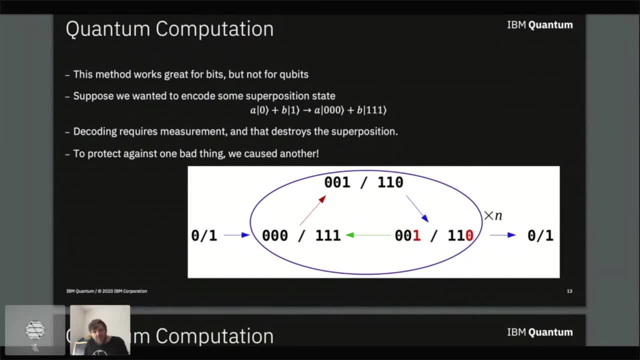 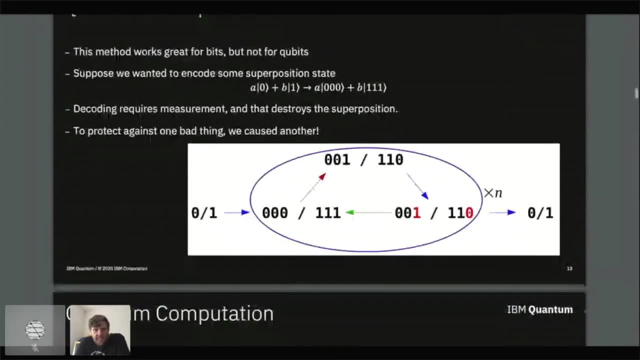 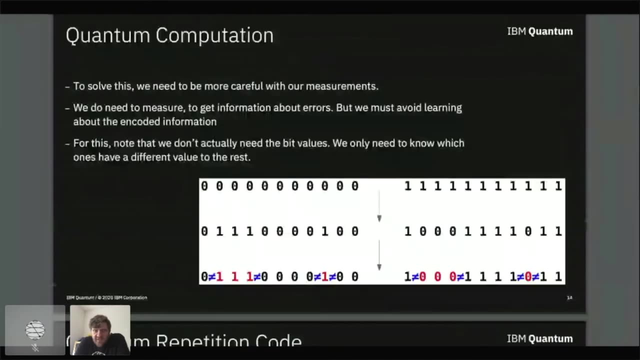 It's flipping when we don't want them to. We actually caused another bad thing, which is the collapse of the superposition. Okay, Um, yeah, so I just thought I'd stop here and ask if there's any questions so far, 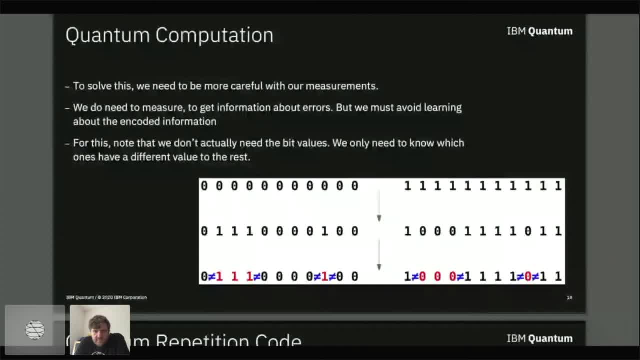 Yeah, we've got a few questions that I think are pretty relevant to what we're talking about right now. one- and you may get to this later- but since errors appear due to hardware, won't the error correction algorithms be different for different hardware? 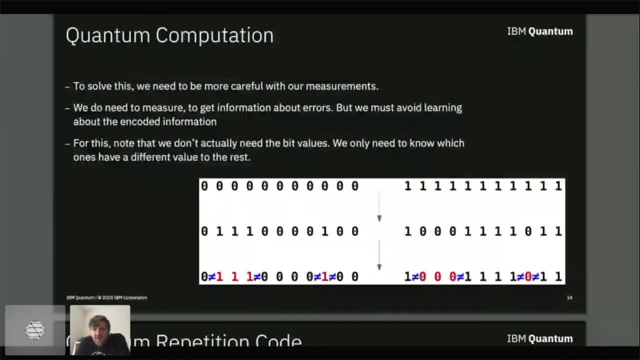 Um, well, that's a good question. Um, now, over the years, we working on error correction have been pretty much just as abstract in our thinking as people who work on algorithms. The only difference is that they assume that there's no errors and we assume that there. 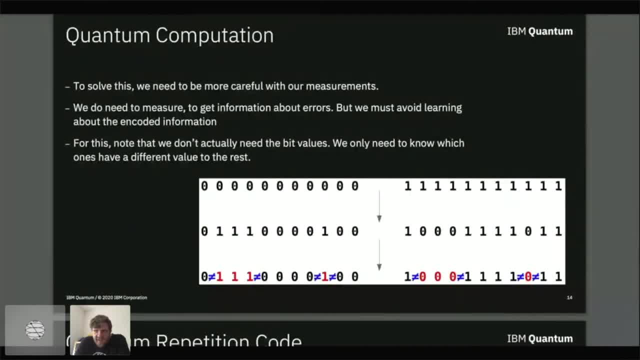 is uh, and the errors that we assume are usually nice toy models of, uh, easy to understand algorithms. I always think of it as a little gremlin sitting next to every qubit flipping, flipping a, rolling a dice or something, deciding what to do. 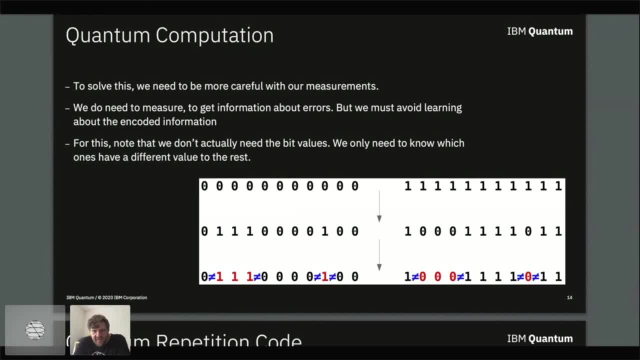 And if it comes up the wrong value, hitting the qubit with a, with an X or Y or Z. this is the sort of error model that we've traditionally looked at And for that it's well. at that level it's the same whether you think of it in terms 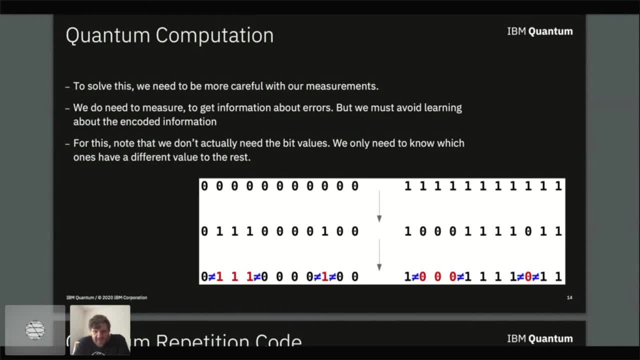 of spin qubits or or superconducting qubits or whatever. uh, other than that, I think there will need error correction, will need to be tailored to the hardware to some degree. But, um, also, the way error correction works is it's, it's very- it's- kind of agnostic. 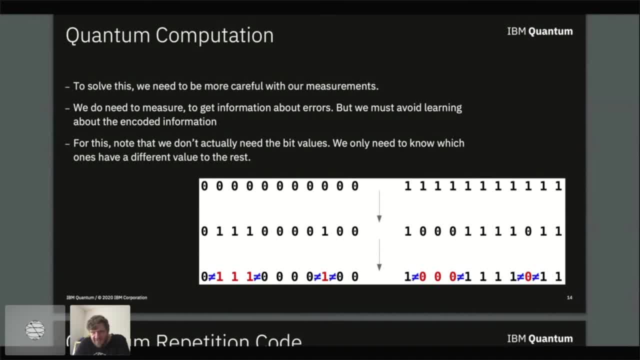 as to the errors, as long as the errors are local, So they act on single Q. it acts on single qubits or small um groups of qubits. then the assumptions of error correction will work. Uh, but if you want the best performance you will have to tailor it to the device to 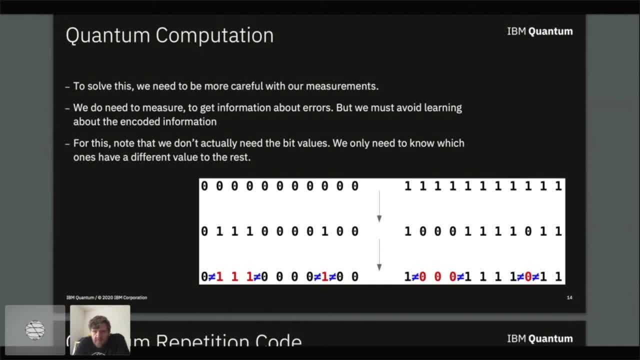 agree, Awesome. And then one more question for now. aside from quantum error correction, are statistical methods used to normalize results, such as reducing columns in the histogram based on the distance to the largest column, or at least calculating the difference? Yeah, So things like that would be called error mitigation techniques. 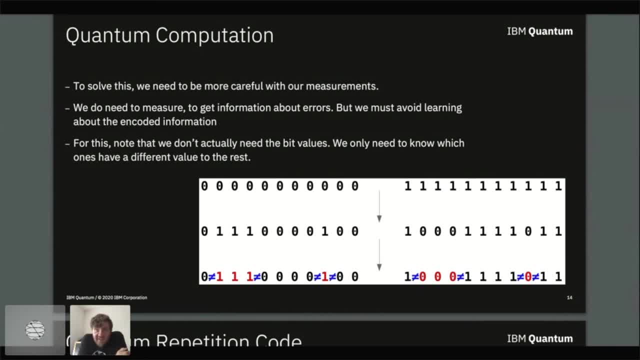 And there is um. if you look in the Qiskit textbook there is also a section on on some of the error mitigation techniques we have there. Uh, such as I keep it. imagine if you've got a, a single qubit, you could prepare it. 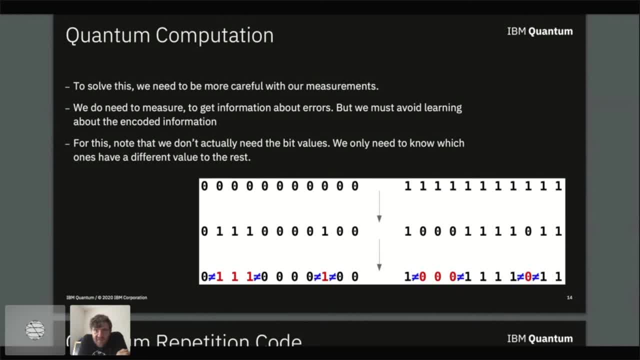 in the zero state and then run many shots to see what the histogram looks like, And so it will be lots of zeros and a few ones, and then you know: well, that's okay, That's what. uh, that's what a zero looks like in terms of the histogram. 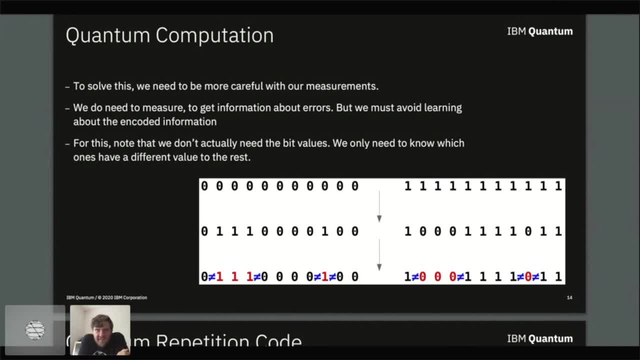 And then you do the same thing for one- they'll see what a one looks like. And then you do the same thing for anything arbitrary And you can find kind of look at the histogram you get from that and think, well, given that. 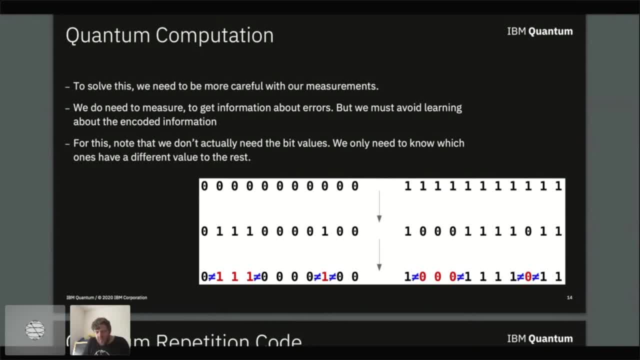 I know what What a zero histogram looks like and given I know what a one histogram looks like, what can I deduce about what this histogram should have looked like? So you can do- there's all kinds of error error mitigation techniques that we can- we. 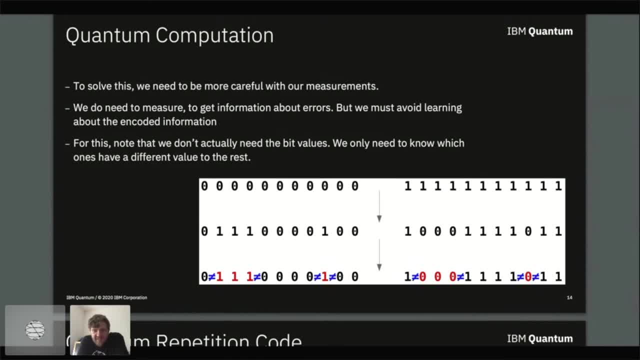 know already and I'm sure we'll develop more, because this is this is more relevant to the next decade than quantum error correction. arguably Awesome. I'll give it back to you to continue with your lecture. Thank you, Um, okay. 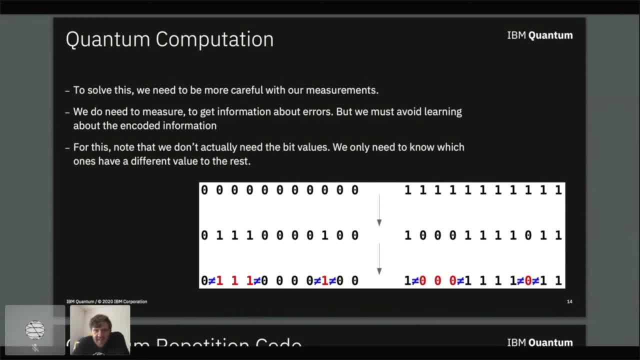 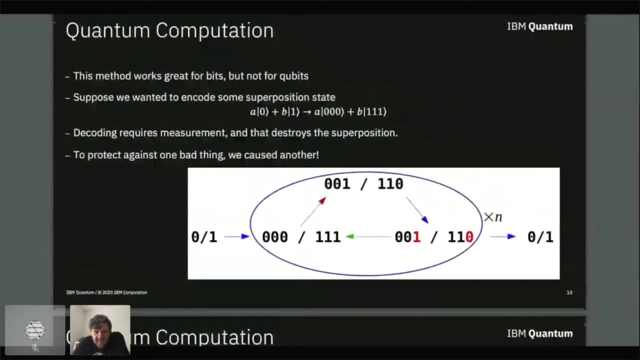 So we have a problem? Okay, So we have a problem, And our problem is that we need, you know, we couldn't have identified this error without looking at our qubits and working out, um, where the error was. uh, but looking at our 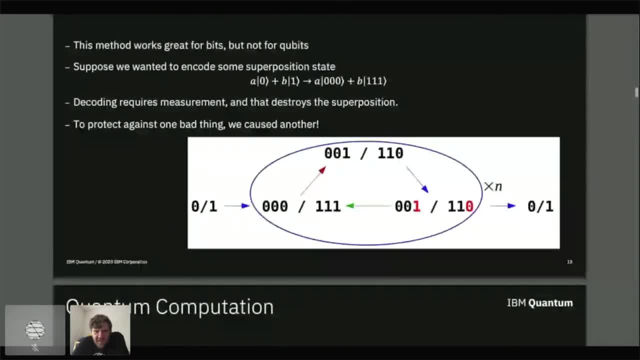 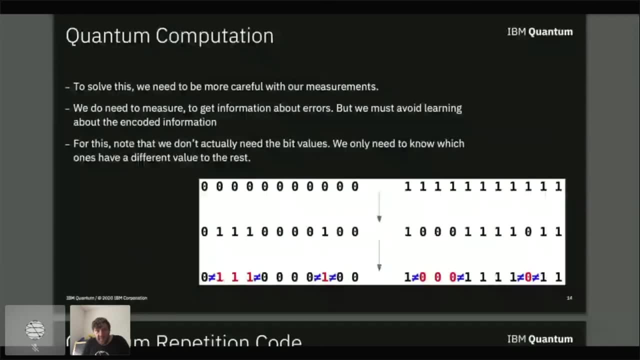 qubits destroyed our superposition. So how do I, how do we look at our qubits without looking at our qubits? How do we measure without measuring? Um well, we just have to be careful about what we measure We are. there's not no law against us measuring in some form. 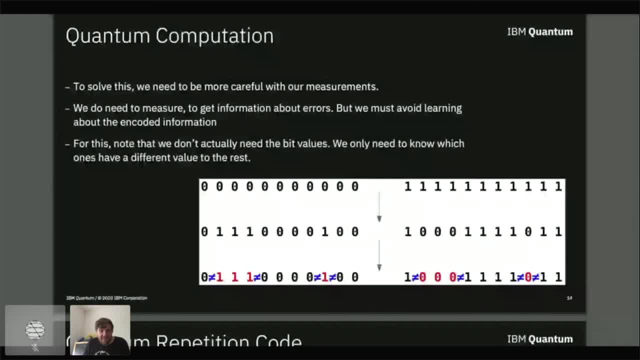 There's no law against us. We are extracting information about the errors, but we just must not extract information that causes the superposition to collapse. If we ask a qubit, are you zero or one? it has no choice but to choose and collapse. 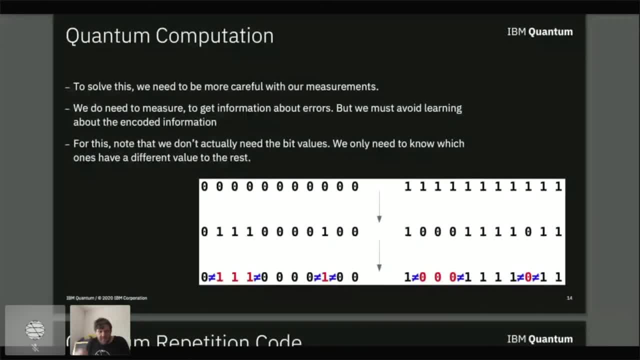 a superposition, Um, but if we, if we ask a group of qubits some other question, then it might not cause all of the qubits to collapse into particular superposition. So let's go into this in a little more detail. 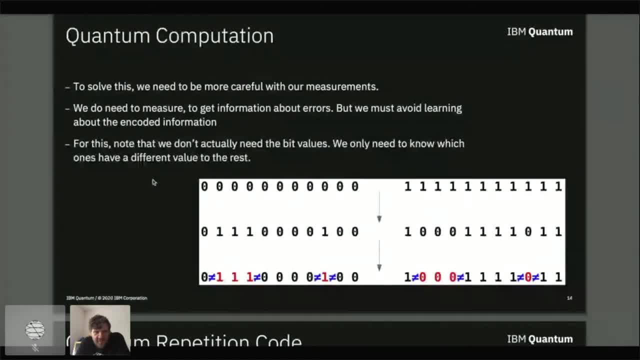 Um. so yeah, We do need to measure, but we have to avoid learning about the encoded information. So let's look and look at an example where we have here, um, a repetition code with a one, two, three, four, five, six, seven, eight, nine, 10, 11 repetitions. 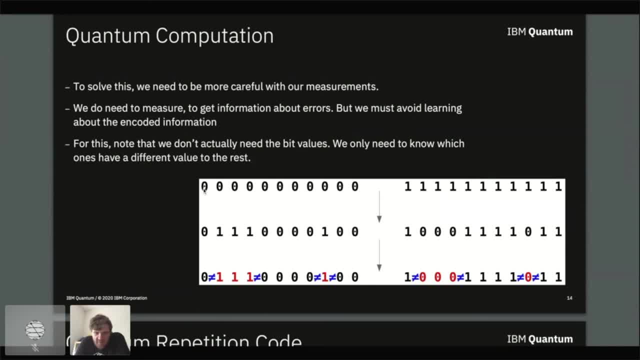 Uh, so whether we, if we encoded a zero, it would be this series of 11 zeros, If we encoded a one, it would be this series of 11 ones. Now, let's assume that errors happen on a particular set of qubits. 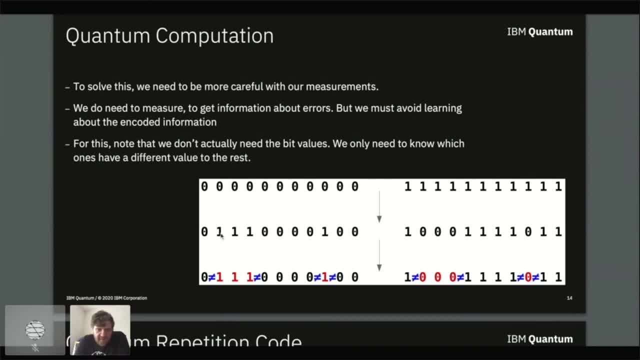 So you can see the ones that are ones, um, affecting the zero, Um, if that makes any sense, these ones that are flipped in the line that should be all zeros, the ones that are flipped to ones. that's where the errors have happened. 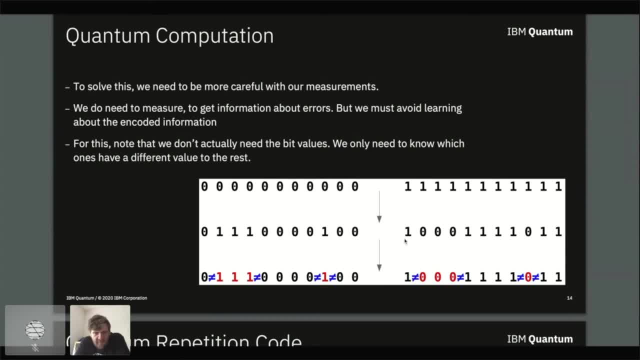 And if you look on the line, that should be all ones I've. I've made it so. errors happen in exactly the same place there, Um, so that, uh, so we're, we're, we're having the same errors compared across wherever they're. 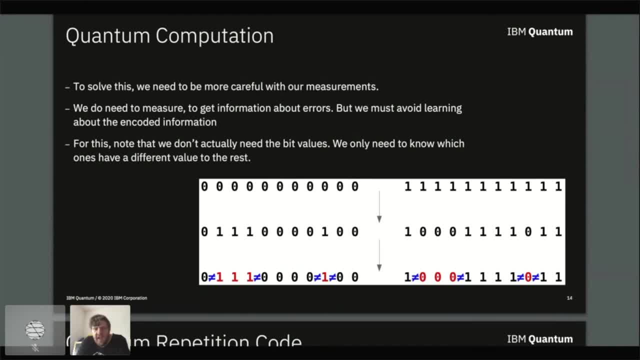 encoded as a, as a zero or as a one, And obviously, if we were to look at these values, we would see that those ones where the error has affected it are in the uh, are not the majority. So the majority voting would disagree with them and say that they're probably the ones. 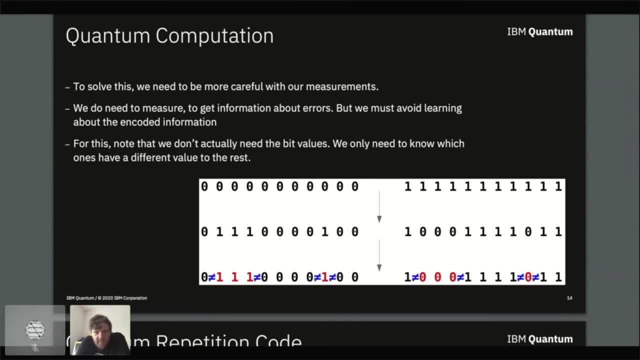 that are. that are the errors. Um, but let's not do that. Let's instead some go along and look at each pair of qubits along the line or bit value, uh line, and ask: are they the same or different? now, 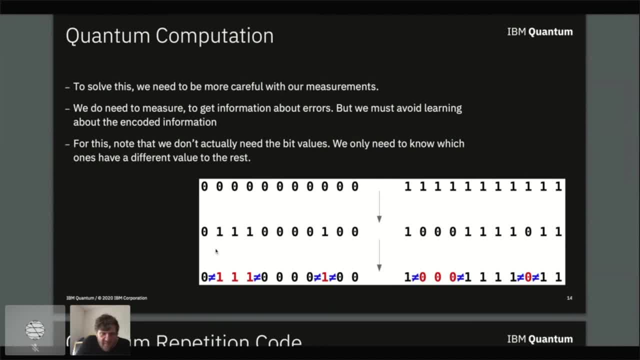 I asked this before, but I said I'll ask again. can you actually? can you see my pointer, or can you only see when I highlight things? We can see your mouse and we could see when you highlight things. Okay, The fact that you can see my mouse makes things a lot more easier. 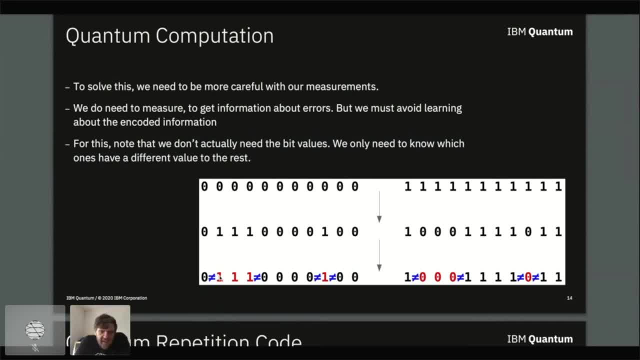 Uh. so if you, uh, if you look at a pair of qubits- sorry a bit- if you look at a pair of bit values, uh, this is what you see. Uh, this is what you see. This is what you see. 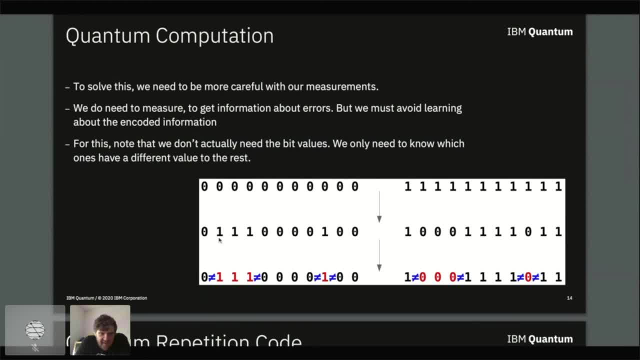 Uh, this is where I highlighted, and you could see from this precision ratio that you can see the difference. bem גати, the same same, same, same, same, same same. And similarly, even though they're a different value over here, still these are the same. 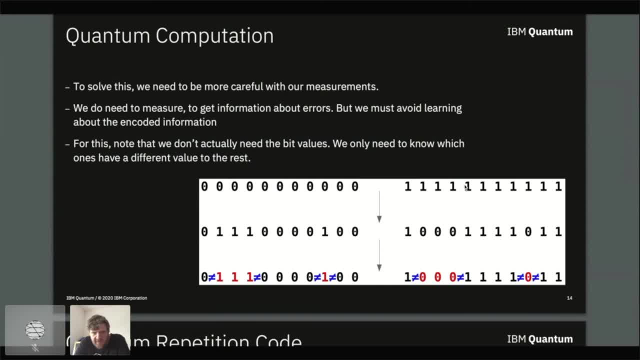 value as each other. These are the same with each other and the same and the same and the same. So a signature of everything being good is that if you look at these pairs of values, you'll find that they always agree with each other. 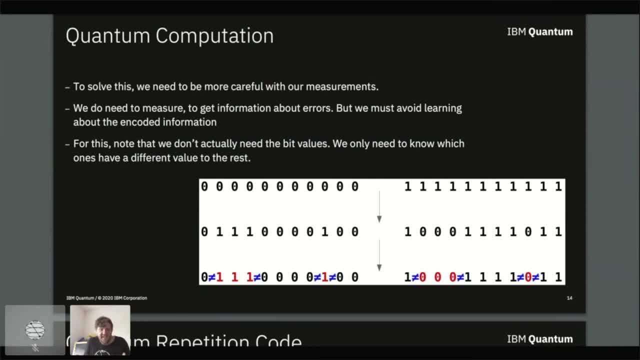 And of course they should. This is the repetition code. You're repeating things. They should agree with each other And then, if we see a single error in the middle of nowhere, here we find that this is different from both of its neighbors. 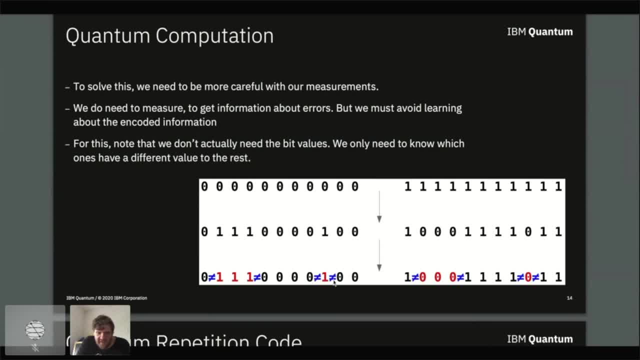 And so the fact that it is different from both of its neighbors. well, seeing any of these two values being different is a signature that there is an error somewhere, And the fact that it's different from both of its neighbors is a fairly strong indication. 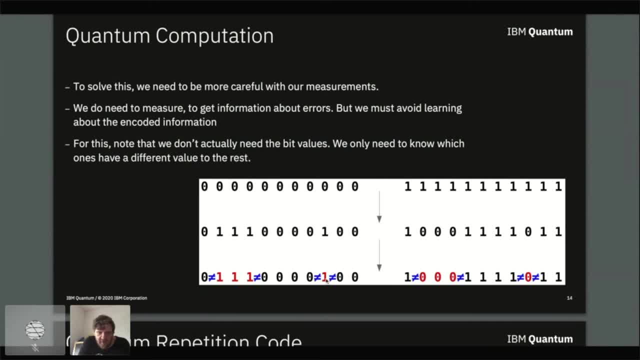 although not conclusive, that this is probably the one that is in the wrong. Similarly, we can find that these are different, but these are the same and these are the same and these are different and same same, same, different, different, same. 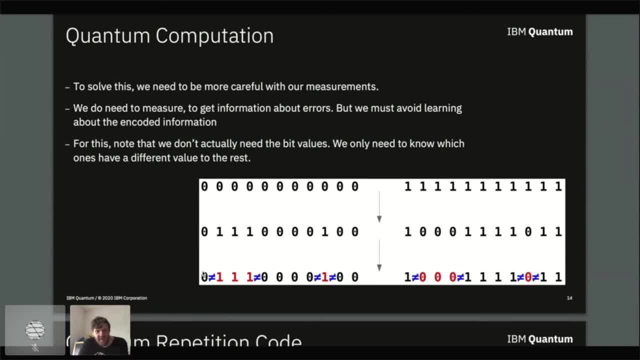 So, knowing that there's, If there's only two values, we can form these into two groups. We have this one, which is in one group, and then this one is in another group because it's a different value. Since these are the same as this value, they're also in the second group. 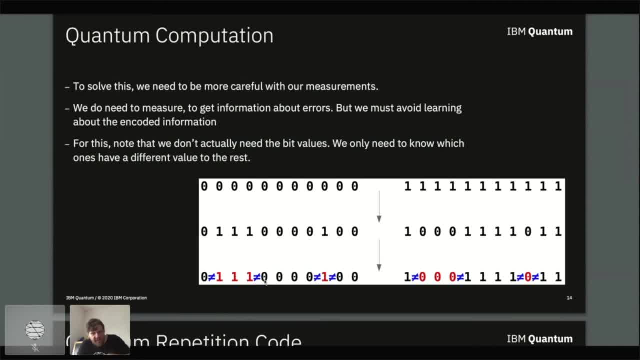 And since this one is different from that one, we know that we must have gone back to the first group, But these all belong to the first group. This is again in the second group. These are back to the first group. So even by just 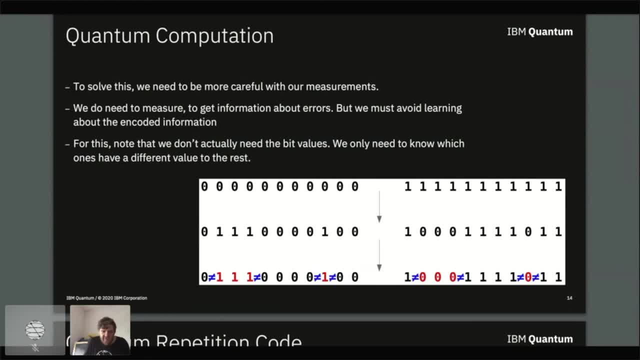 Knowing whether these values are the same or different. without knowing what the values actually are, we can still do majority voting. We can still split it into two groups and find that one is in the majority, one is in the minority, and assume that the majority are the ones that haven't had the error. 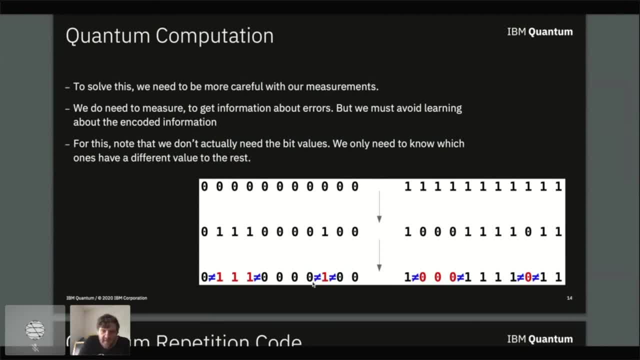 and correct accordingly. So this And the exact same process would have worked exactly the same if we had encoded a 1, because it doesn't care whether we've encoded a 0 or a 1. Because we are just looking at whether values are the same or different. 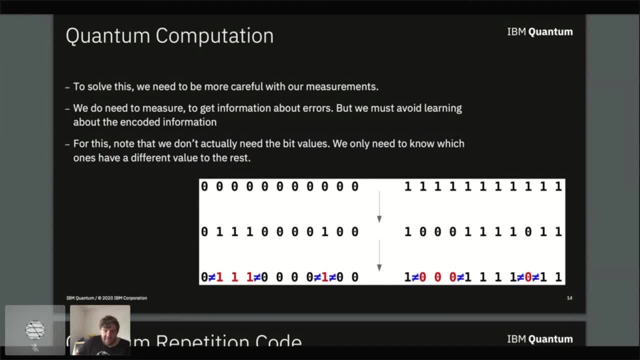 We're not looking at what those values are, We're just looking at their relative values between each other. So the insight here is that we can still do majority voting without actually knowing what the bit values are, And we do that not by looking at the bit values. 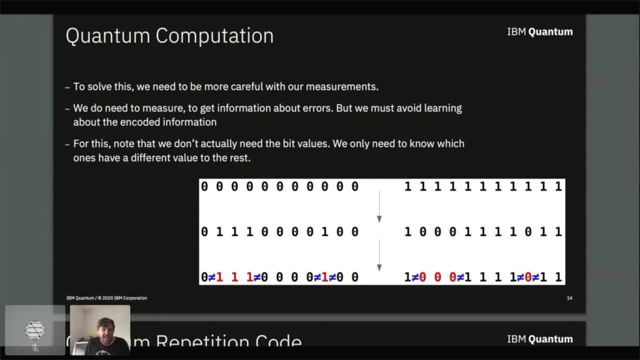 because that would, of course, have told us what the bit values are, but by instead only extracting the information about whether they're the same or different. So you bring, You put your two bits together and you don't look at them and you say: 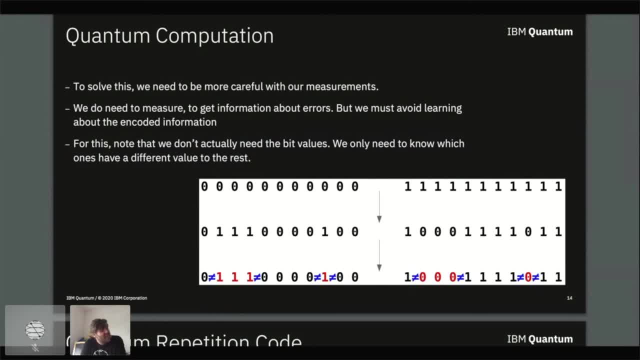 I don't want to know what you are, I just want to know: are you the same or different? And then they'd say we're the same. And you'd say, oh, thank you. And then you go along querying all of these. 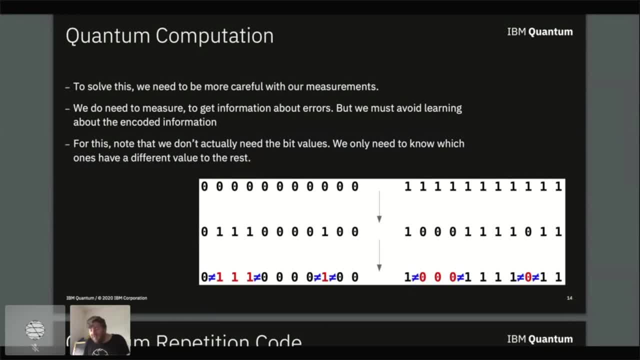 And with that information you would be able to do the error correction without knowing any of these values. And this would mean that even if you've got a superposition of lots of 0s and lots of 1s, which became a superposition, 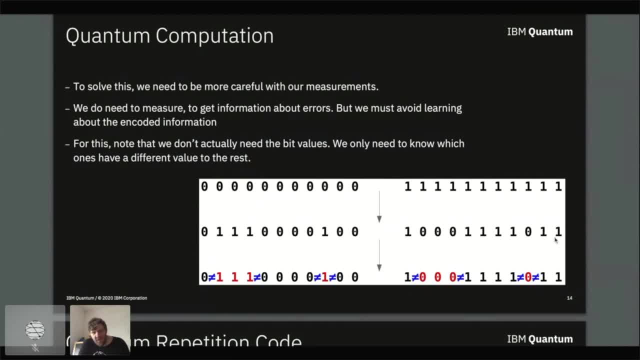 of this thing and that thing when you had errors. then when you ask a pair of qubits- are they the same or different? then the outcome does not disturb the superposition. It doesn't care about the fact that there's a superposition. 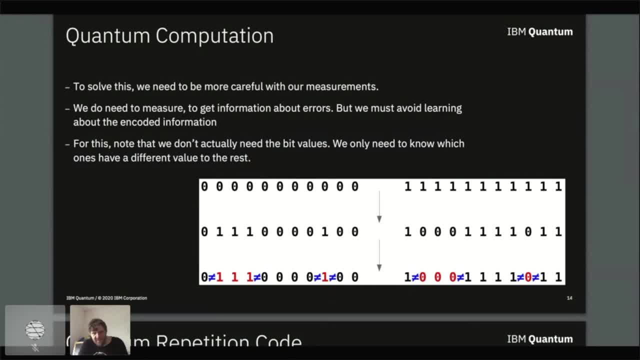 It will tell you exactly the same results as if you had just done a 0 or a 1.. So this is the information we need to extract. We need to do this thing where we're going to take two qubits and ask in the 0-1 basis. 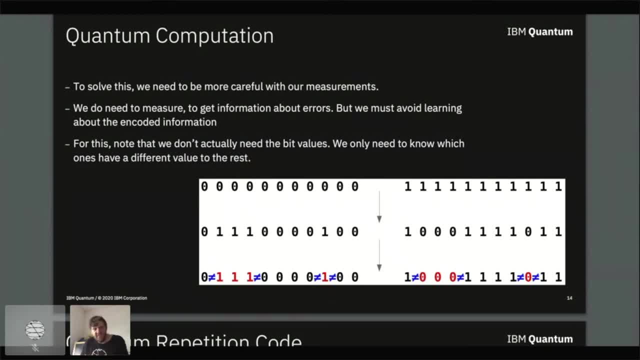 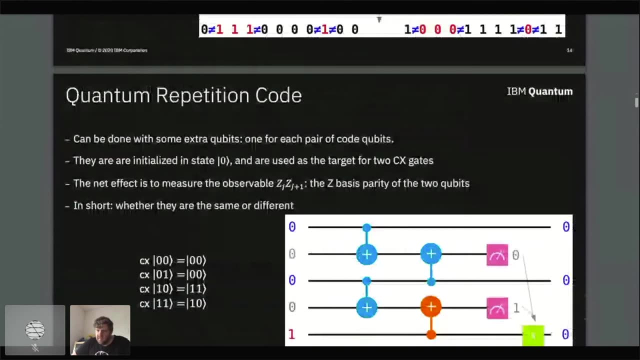 are you the same or different- and extract that one bit of information- same or different- without actually looking at what they are. Okay, So how do we do that? So I think this is probably the point where I would probably pick up my pen. 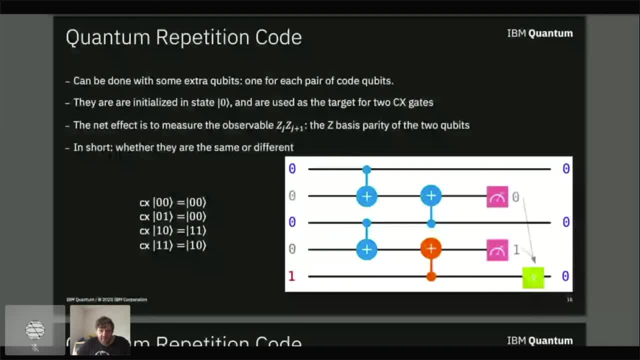 and start doing stuff in a written way, But because I'm doing it as a PDF on a browser, probably I'll have to stick with not doing that, But I think it should all be pretty much the same. anyway, My handwriting is atrocious. 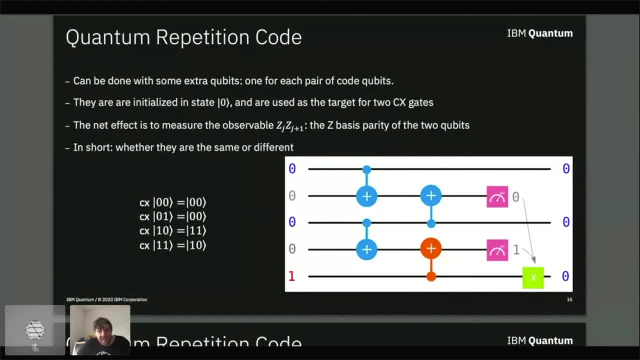 and that's why I do things on PowerPoints mostly. So you're probably getting away lucky without having to look at that. Okay, So the way that we can do this, this task, which is to take a pair of qubits and see if they're the same or different, 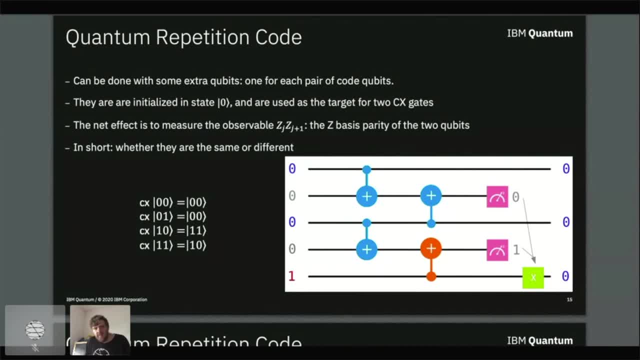 without otherwise extracting any information. we can do this by taking an extra qubit. So for every pair that we want to ask this question, we take one extra qubit. So we have an example here where we have three repetitions. These are the colored values here. 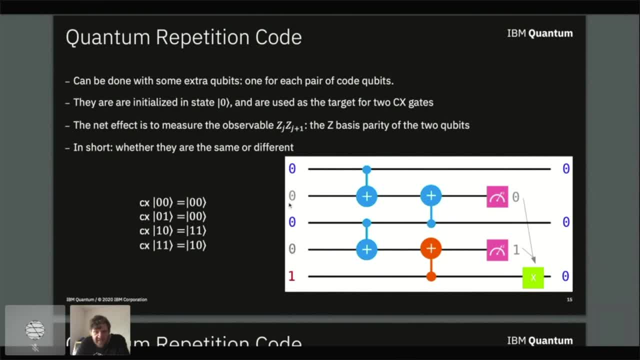 And then we have two extra qubits, which we usually call ancillars, which are the gray values here. So if we want to know whether these two are the same or different, then what we do is we use a couple of controlled, not gates. 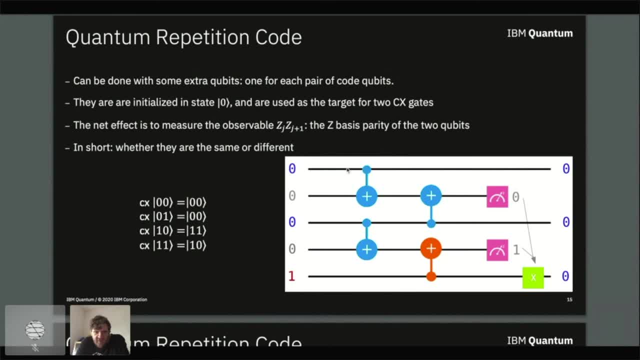 So the first controlled- not gate is controlled- is controlled on one of the qubits we want to compare and targeted on the extra qubit, the ancilla. The other is controlled on the other qubit we want to compare when we're comparing this pair. 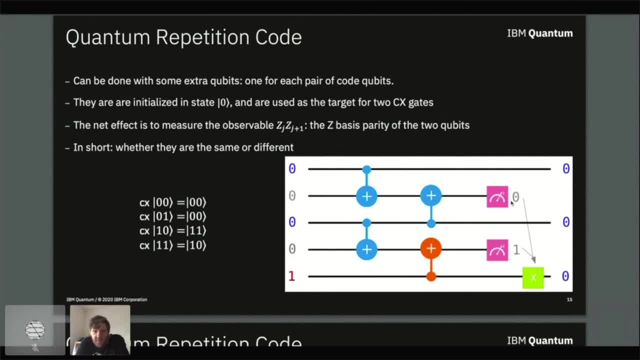 and targeted again on the same ancilla. And then what we do is we measure the ancilla and we get a result of either zero or one. So what is the relevance of that result? Well, let's see. Let's consider the case where these are. 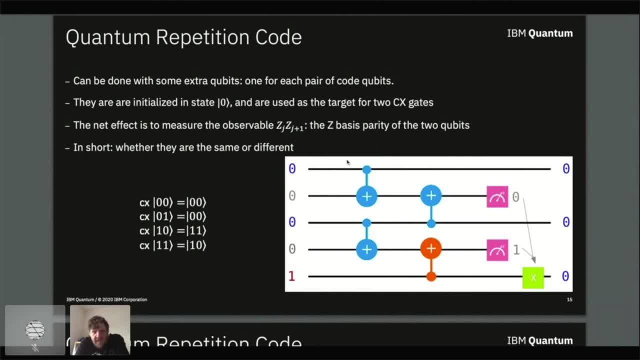 both zero, which is actually what we see here In this case. well, a controlled- not controlled- on a zero does nothing, So this does nothing. This one is also controlled on a zero, So it also does nothing. So our ancilla, which was initially zero, 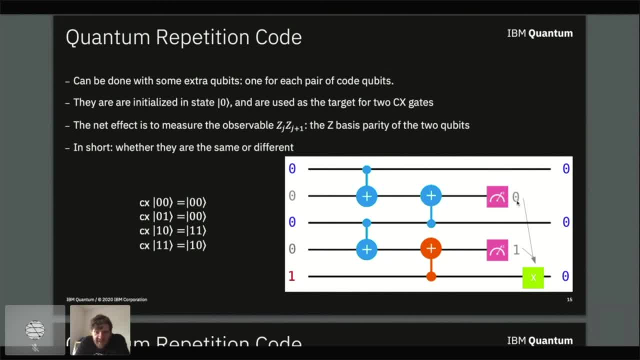 is still zero at the end, And when we measure it it tells us zero. So in the case where they are both zero, we get a zero out here. Now, if they were both one, so if this was a one and that was a one. 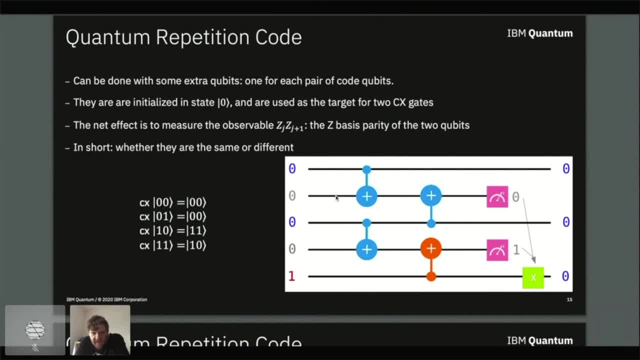 then what would happen? Okay, so this is still initially zero. It goes along. It meets this controlled not. What does this controlled not do to it? Well, a controlled not. we can tell the story that it looks at the control and looks at whether it's a zero or a one. 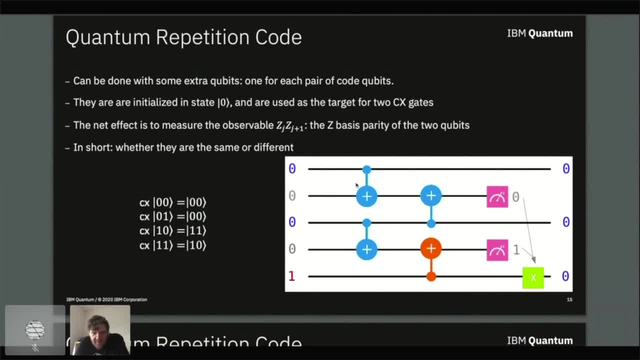 If it's zero, it does nothing. So that's exactly what we just talked about. If there is a one here, however, it will flip, It will do an X, It will flip this bit, It will flip this zero into a one. 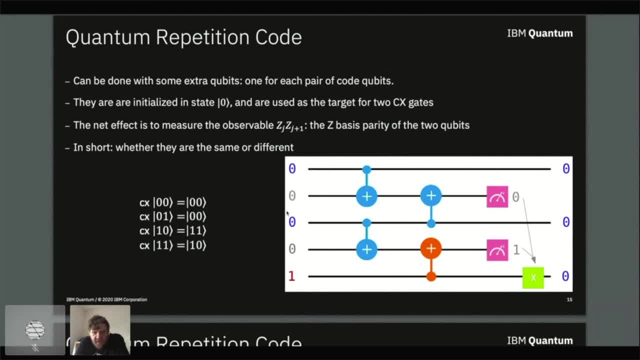 So in the case that we are comparing two ones over here, then this ancilla gets flipped from zero to one after this first CNOT, But by the exact same effect by the second CNOT it gets flipped again back to zero. So in the case that these two are both one, 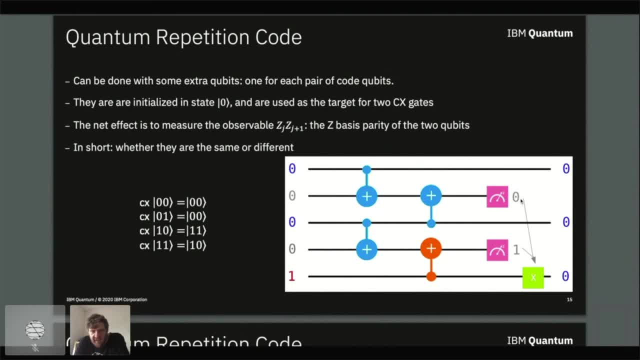 we have that. we measure a zero at the end. So whether they're both zero or they're both one, this measurement does not know, does not care. All it knows is if they are the same. it gives a zero. Now what about when it gives a one? 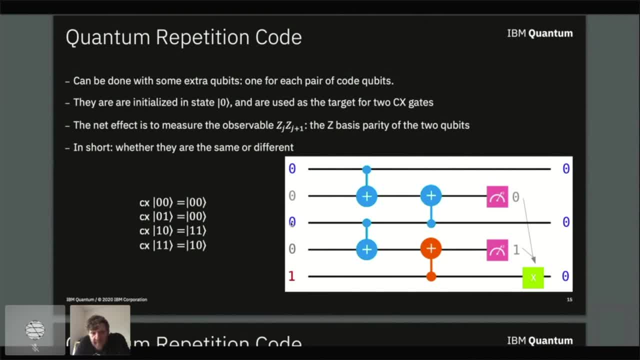 So we see this example at the bottom here. So if you have, if they are different, so if this is a zero as it is and this is a one, then this CNOT control on the zero will do nothing. The CNOT control on the one will flip the ancilla. 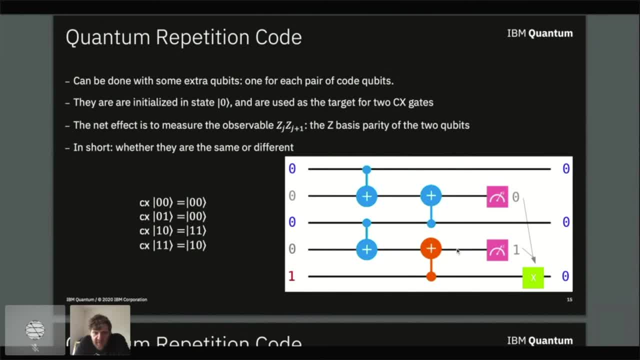 So the ancilla gets flipped exactly one time, flipping from zero to one, and so the answer you get at the end is one, And it doesn't matter if it was zero one or one zero that you're comparing. In either case, 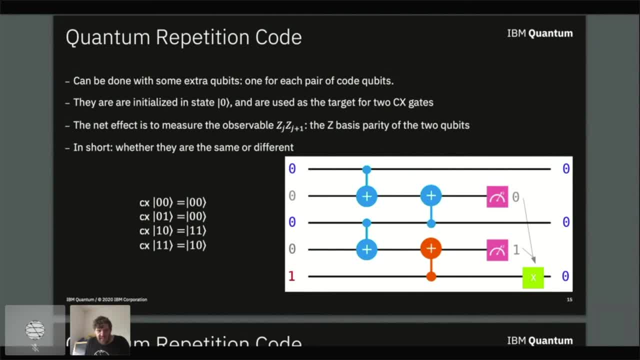 where they're different, you get a one at the end. So by introducing this extra qubit and by doing these controlled CNOTs, we have found a way to not measure the qubits themselves, not get any information about what their value is. 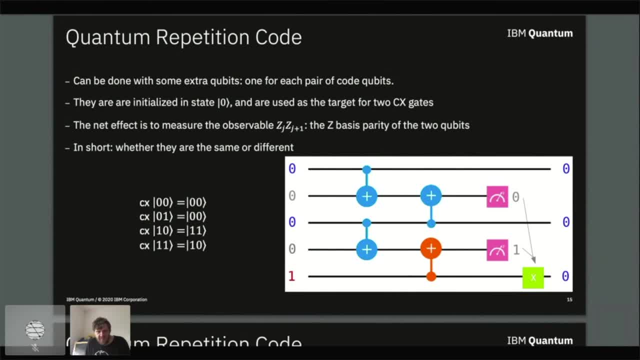 except that we are comparing whether they're the same or different. We want to know: you could be zero, you could be. so we take a pair and we say: well, you could be zero, zero, or you could be one one. 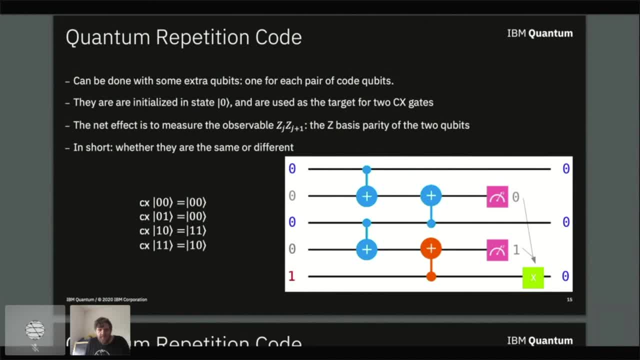 or you could be some superposition of that. We don't care, We just want to distinguish that from the case where you're zero one or you're one zero or you're some superposition of that. Can you distinguish those two cases? 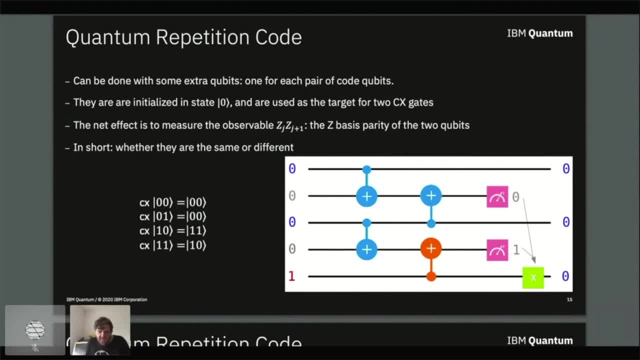 of you being some sort of same or some sort of different, And by measuring the ancilla, that is exactly the information you get. Zero tells you that they're the same. One tells you that they're different. And by taking that information, 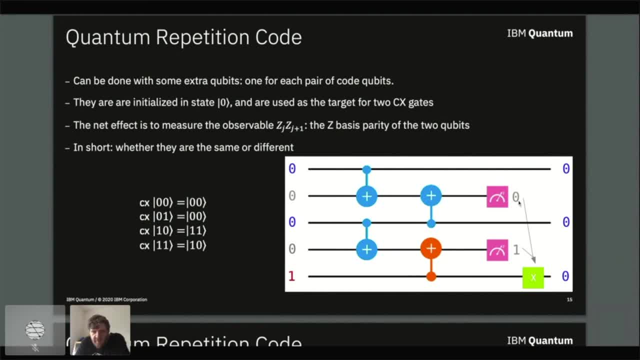 we can get some information about what might have happened. So by saying that these two are the same and these two are different, by combining that information, we can say: well, okay, that means that this qubit is the odd one out.